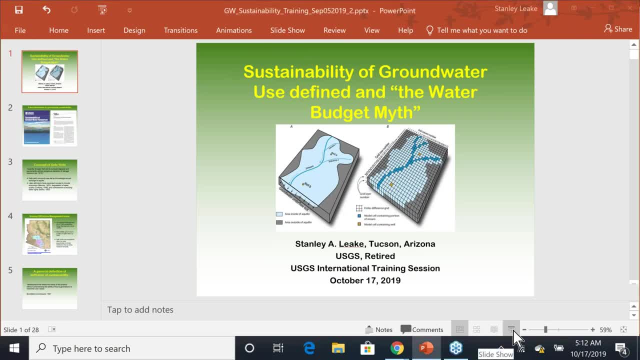 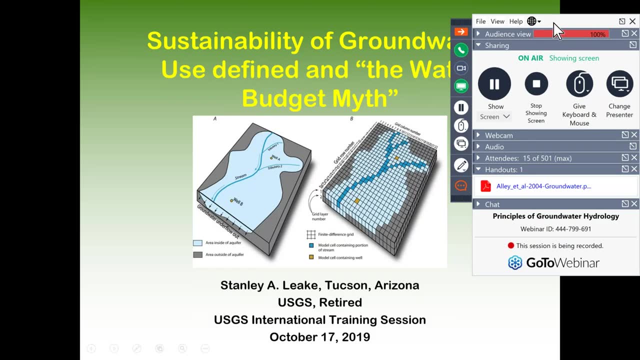 The broadcast is now starting. All attendees are in listen-only mode. Good afternoon everybody. This is Clara Bocchino, from South Africa, on behalf of the Big Data Analytics and Transboundary Water Collaboration for Southern Africa, of which the Sustainable Water Program is a partner, and USGS, the US Geological Survey. And this is the final. 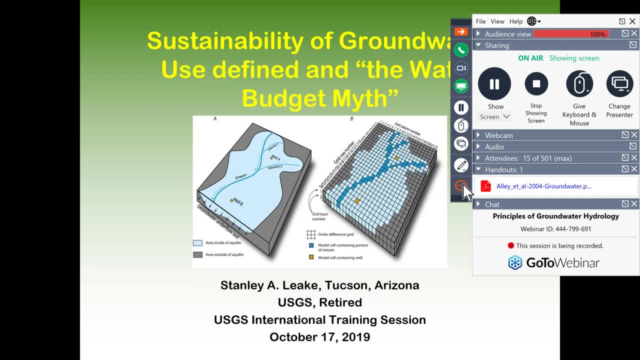 webinar that we do with USGS and it's with Dr Stan Leakey who's going to talk to us about sustainability of groundwater use. For now you are all muted, just so that the presentation can run smoothly and we don't have any background noises. However, we encourage 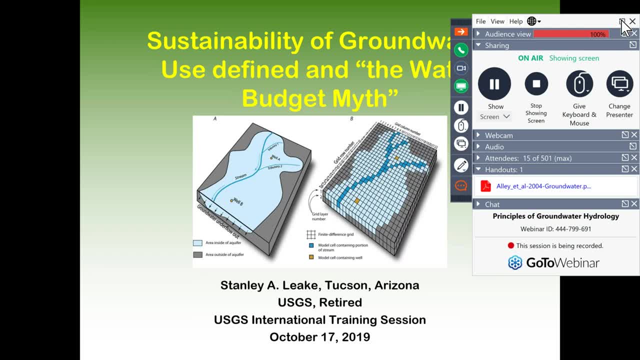 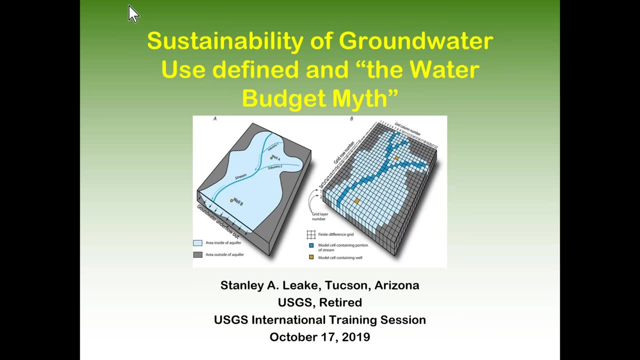 you to ask questions throughout the presentation, and you can do so by using the questions tab on your control panel for the GoToWebinar, or you can use the chat mode as well, or, if you really have a pending question that you need to ask immediately, you can just do it. 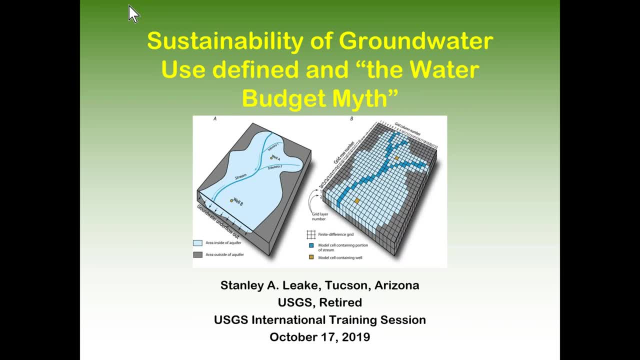 on the GoToWebinar, or you can do a show of hands and raise your hand, So there's different ways in which we can interact with each other during the presentation. As I see questions and I work with Stan, we will sort of make time for you to ask the question directly. 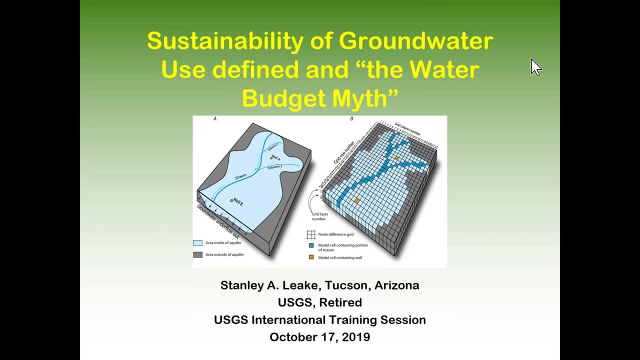 I just want to see what it is before I can give you the voice And then we. otherwise, we're going to have a discussion at the end and if we have enough time, we can do both. Stan, just so you're aware, a lot of us in South Africa are working on a load shedding. 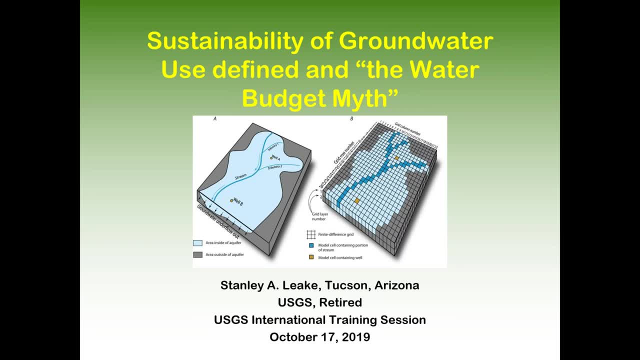 right now. So if people have to disappear throughout the conversation, it's also probably because the electricity ran out. So, without much further ado, let me give the word to Stan And thank you for being here today. I know that we had to reschedule your presentation and so thank. 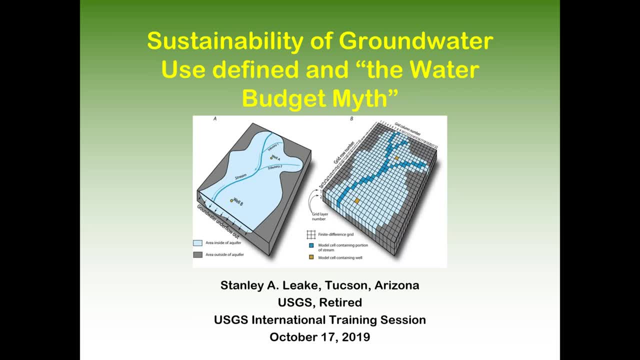 you for making yourself available again, and we're all really looking forward to it. The floor is yours. Thank you. Something called the water budget myth, So I had done some work in this area, although not recently, but I'm going to present to. 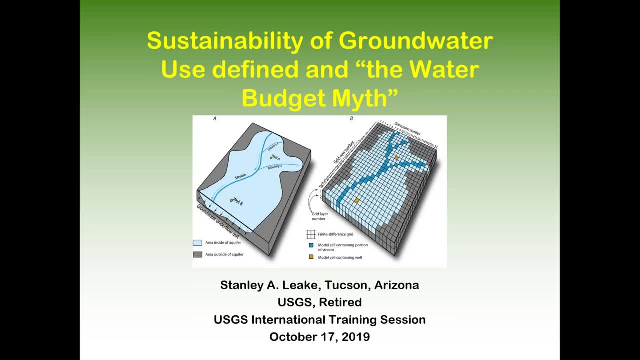 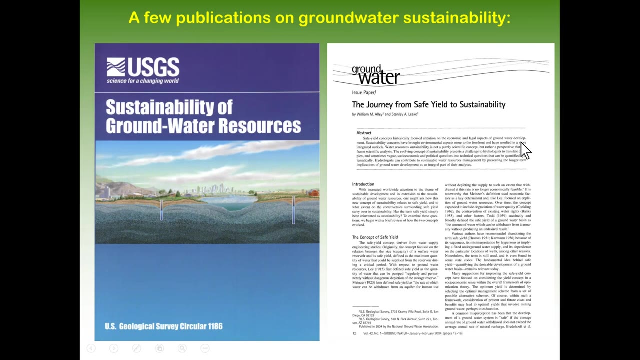 you some thoughts on this And let's see I can get this to advance, Oh yeah, Okay. So I want to refer you to two publications that relate to sustainability Groundwater. The first is the USGS Circular 1186, which you could just Google, that USGS. 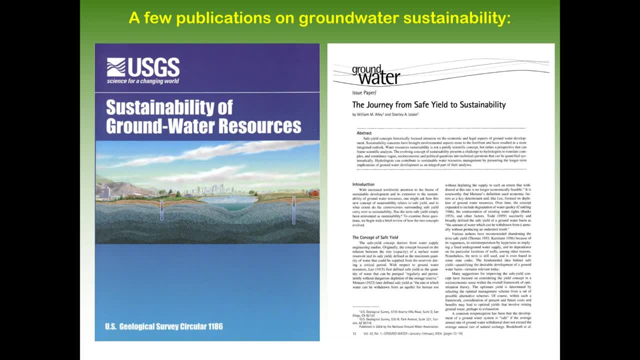 Circular 1186, and it would take you to this report. Another is a journal article that Bill Alley and I did. It's called The Journey from Safe Yield, The Journey from Safe Yield to Sustainability, And I've sent Clara a copy of that that you'd 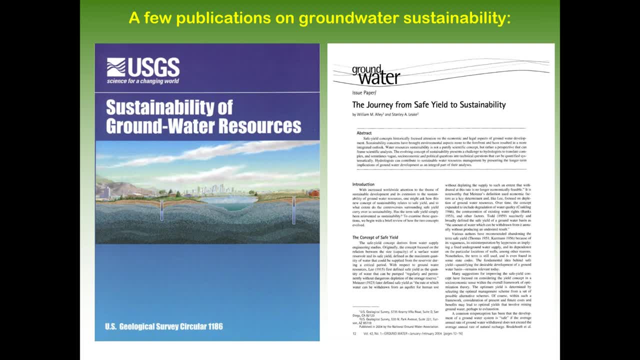 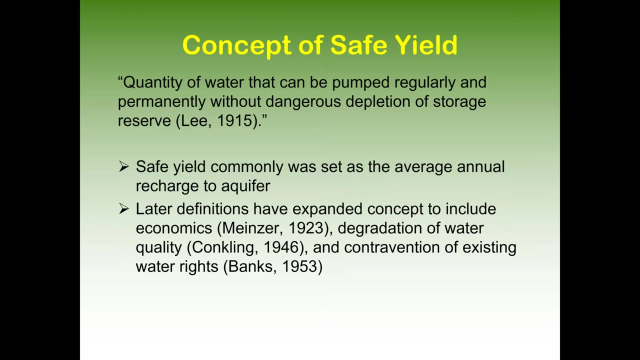 be welcome to take that and read it if you're inclined to do that, And a lot of the material that I got is from in this presentation is from this journal article. So the first concept we have is safe yield And that's a fairly old concept. Alley in 1915 said it's. 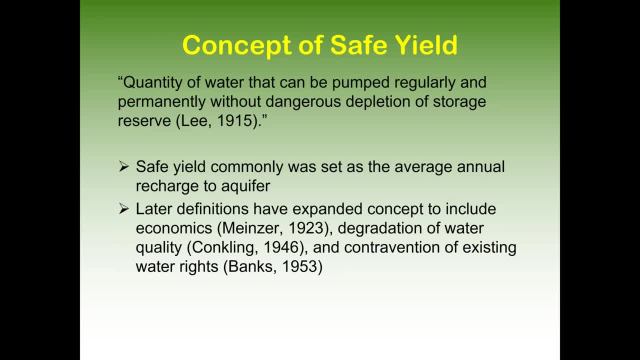 the quantity of water that can be pumped regularly and permanently without dangerous depletion of storage reserve. So fairly basic. It was oriented just towards making sure you don't deplete the aquifer. You still have water in the aquifer aquifer And that was commonly set as the average annual recharge to the aquifer. So 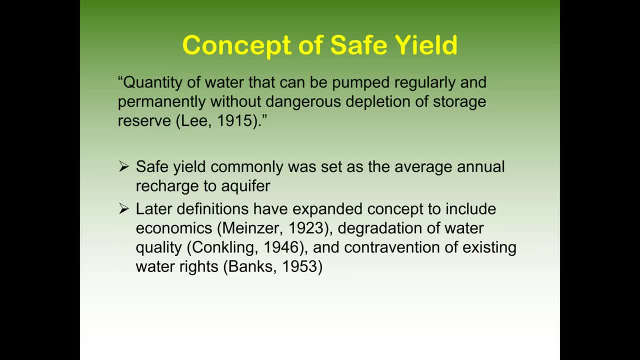 the thinking was that if you pump up to that amount, you're not going to deplete the storage over the long term. And then later, people have expanded this concept to include whether or not it was economically feasible to remove water after some point, or not pumping to a. 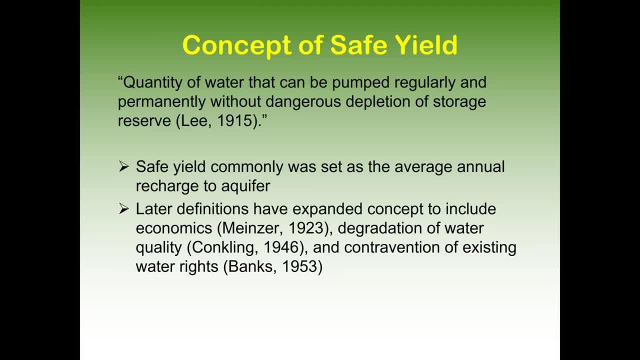 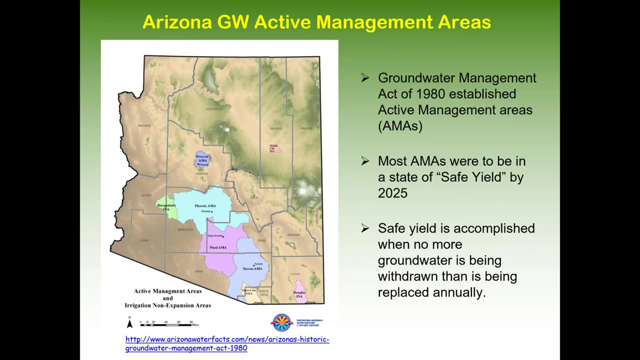 point where you're degrading water quality or you're infringing on someone's existing water rights. So this concept of safe yield has made it into a lot of the water laws in the United States, And I'm just going to give an example of Arizona. In 1980, they passed what's called 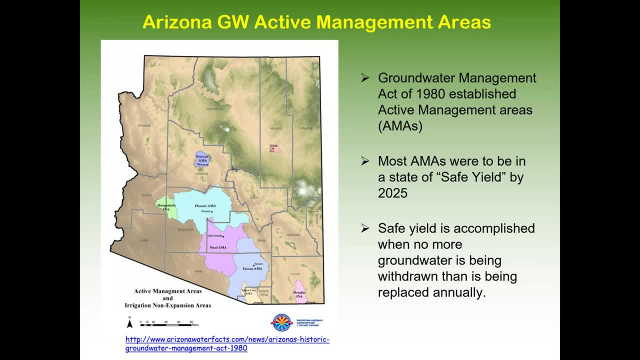 the Groundwater Management Act which – oh, by the way, I live in Arizona, So that's what I'm most familiar with. So they have some very heavily pumped areas. Can you see my arrow? Is that – if I point out things? 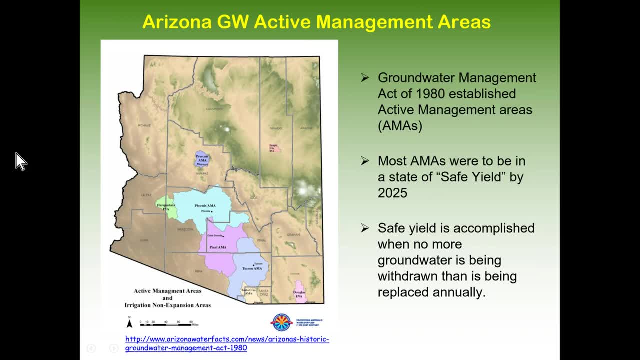 Yes, we can see your arrow. Maybe – let's see, There might be a tool. Anyway, I'm going to – I'm going to go back to the slide. Okay, All right. Well, these large areas of Phoenix AMA, Pinal AMA, Tucson AMA, and then there's one at the 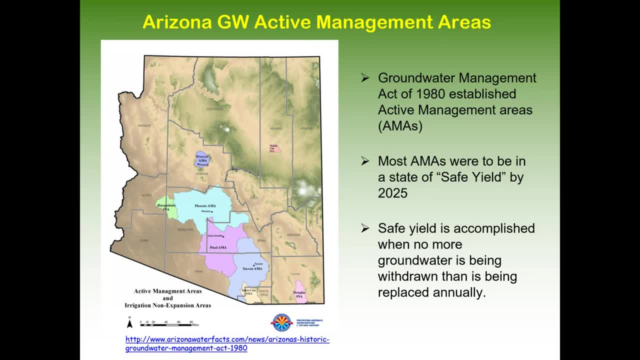 very south, the Santa Cruz AMA. these are heavily regulated areas And under the Groundwater Management Act of 1980, they – Okay Yeah, These AMAs, at least most of them were – it was decreed that they would be in a state. 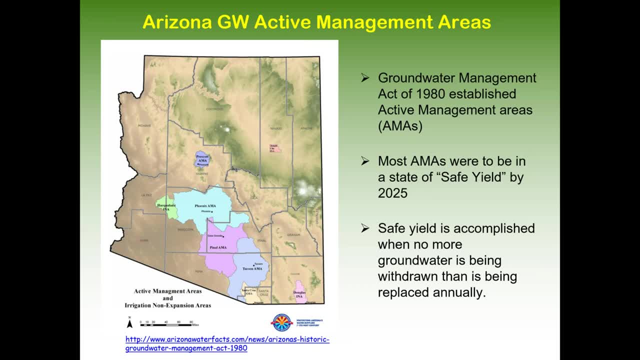 of safe yield by the year 2025. So that was 40 years after this law passed And we're coming up on that safe yield date here pretty quickly And I don't know if you can see that Okay, And I don't think most of them will be, but they define safe yield as the condition. 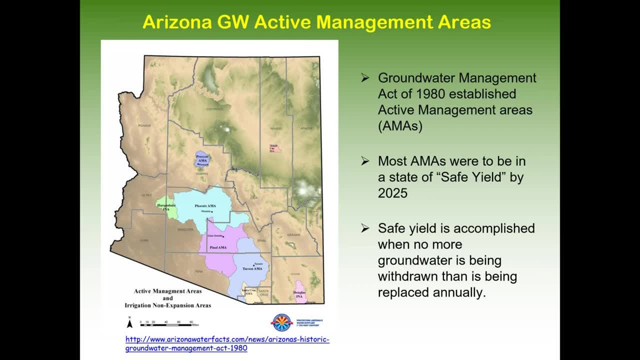 when no more groundwater is being withdrawn than is being replaced annually. So that included both natural recharge to these aquifers and other kind of recharge that might be from imported surface water. Okay, So for instance, when they apply it to the crops, they bring it in from the Colorado. 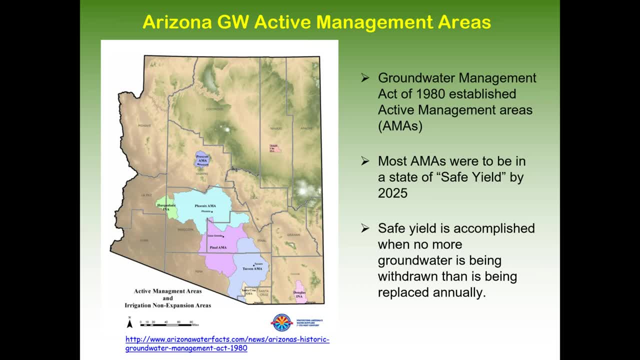 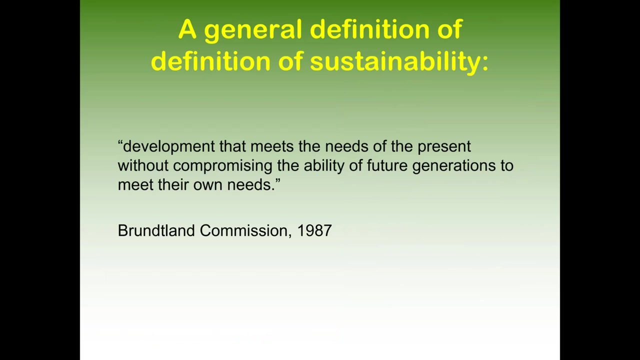 River or something like that, and apply it to the crops. So anyway, that's an example of safe yield making its way into water law. I think other states have it as well. Now, sustainability – you folks probably – I know so much or more about that than I do, but one definition is development. that 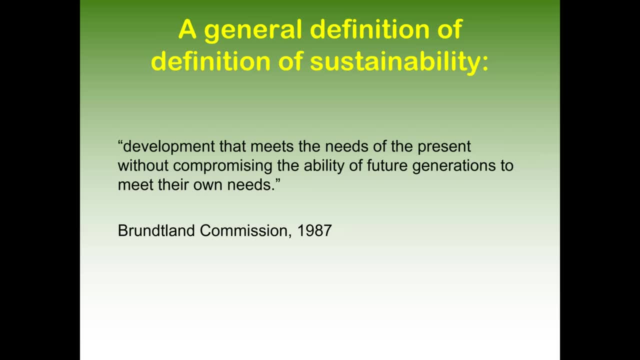 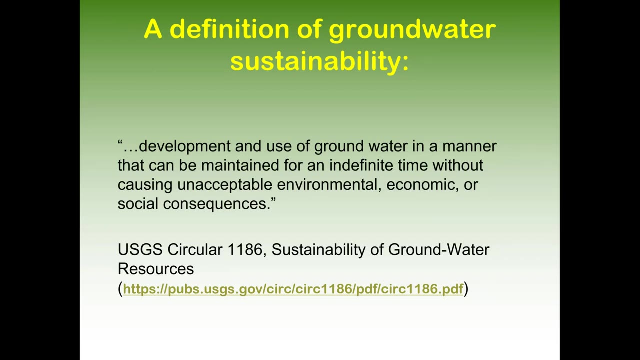 meets the needs of the present without compromising the ability of future generations to meet their own needs. from the Brundtland Commission. And then that circular on groundwater sustainability I had on last – Okay, Okay, Okay, Okay. So that's the second slide. The USGS defined groundwater sustainability as development. 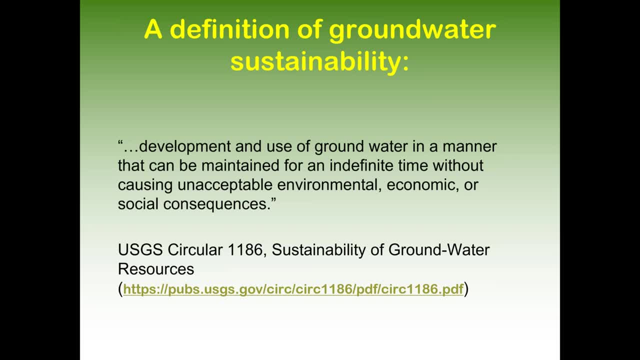 and use of groundwater in a manner that can be maintained for an indefinite period without causing unacceptable environmental, economic or social consequences. And this is interesting because it kind of has this social aspect to it. It's not purely, you know, from a scientific point of view, but what effects of groundwater 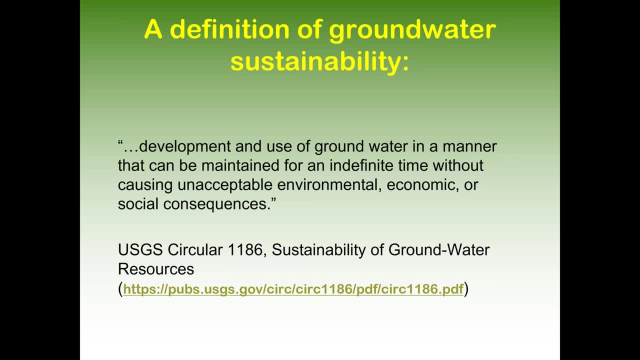 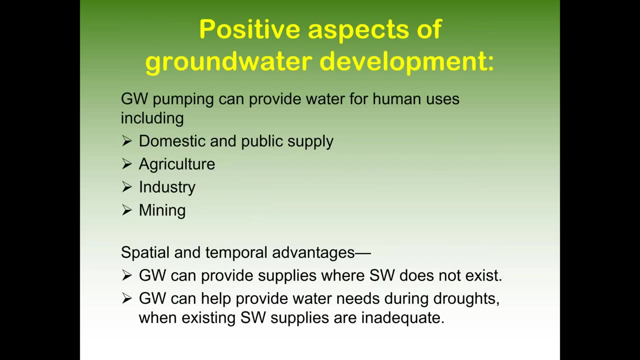 development will society tolerate, or what is acceptable to society. So it's fairly broad in that regard. Now I'm going to talk a little bit more about sustainability. I'm going to talk a little bit more about some of the negative aspects of groundwater development. But I first want 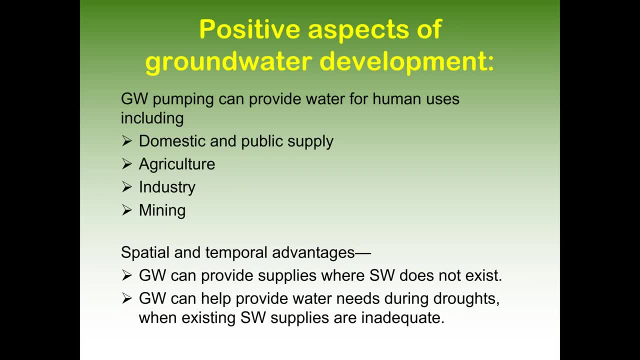 to just mention that kind of the positive aspects, and that is that this groundwater is just a tremendous resource. We use it for so much domestic and public supply, agriculture, industry, mining, And you know it's –, you know it's – you know it's – you know. 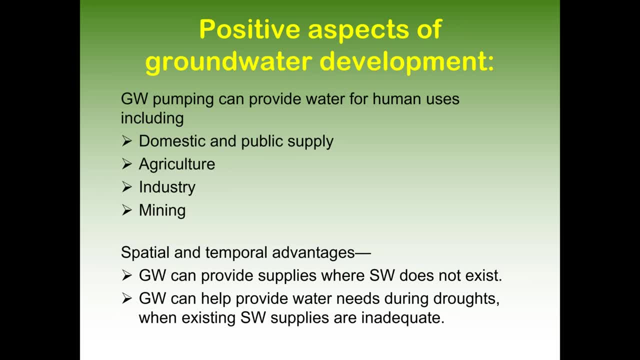 it has some really important spatial and temporal advantages It's – it will provide water for us where we don't have surface water, so it allows us to live in areas that we would otherwise would not be able to live in because of no reliable surface water. that 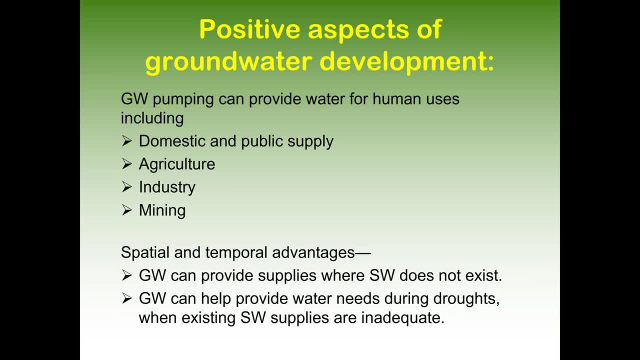 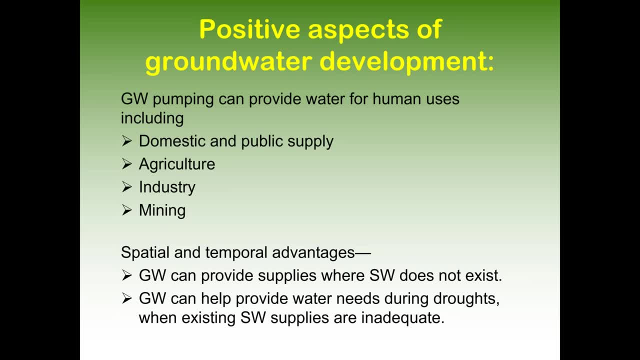 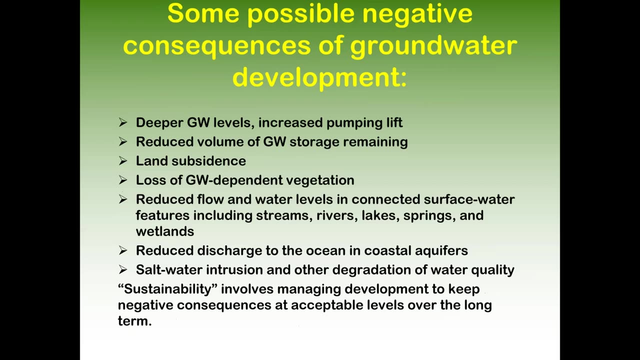 they're inadequate and we can use groundwater, So it is really an important resource. as I'm sure you folks know Now some of the negative consequences When you pump wells and exploit an aquifer: you will have deeper groundwater levels, increased pumping lift. We've had areas in Arizona where 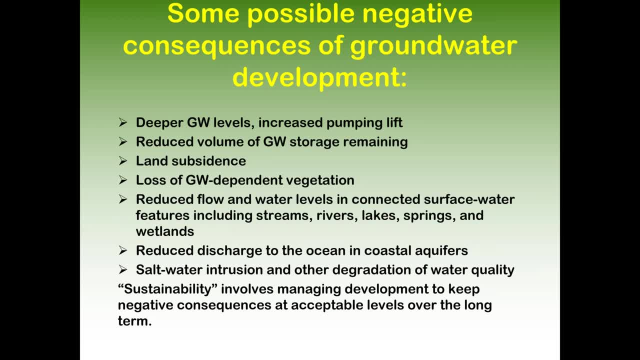 the water table has been drawn down so deep that it's no longer economically feasible to pump water from that depth for safer use in irrigating crops. And then you reduce the volume of groundwater storage remaining. under certain conditions, You could have land subsidence. 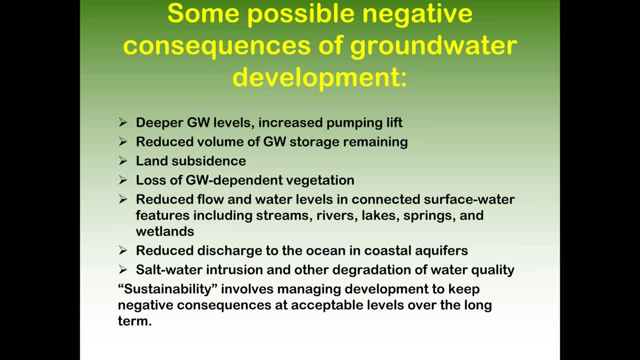 You can lose vegetation that depends on groundwater. So if you have areas where a very shallow water table and you have wetlands, you can lose that by drawing down the water table, by pumping, And then reduce flow and water levels in connected surface water, such as. 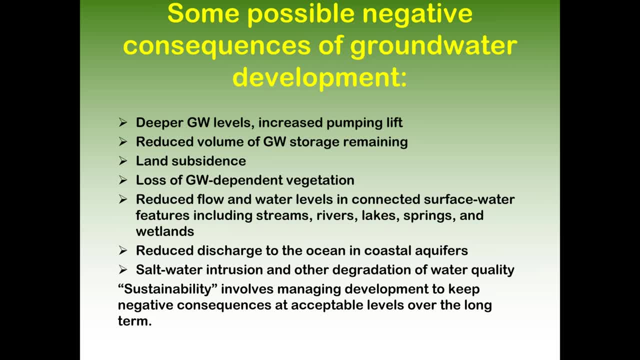 streams, rivers, lakes, springs, things like that. That's a fairly big issue, I think. worldwide Reduce discharge to the ocean and coastal aquifers. That's kind of an unseen effect, I don't – there could be some negative consequences. 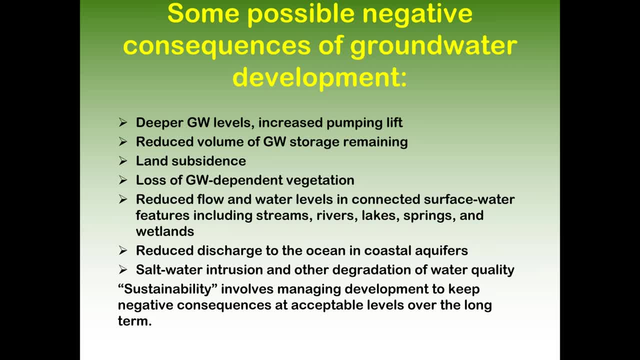 of that. I don't live in an area with coastal aquifers, but maybe some of you know about that. But we do have a lot of areas in the US where in the coastal aquifers the pumping causes saltwater intrusion or maybe what we call upconing of saline water from deeper. 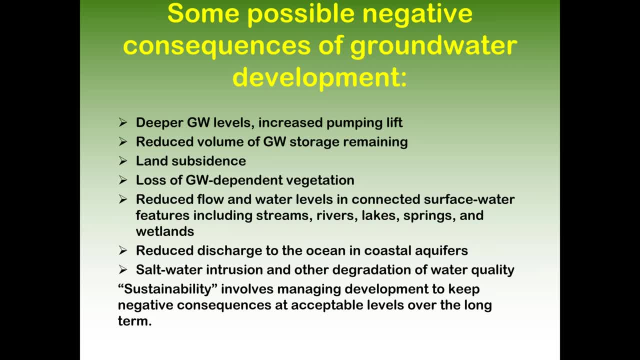 depths below the wells as you pump a well, And our thought is that sustainability – I'm not sure if that's a good word, I'm not sure if that's a good word. I'm not sure if that's a good word, But sustainability involves managing development to keep these negative consequences at some. 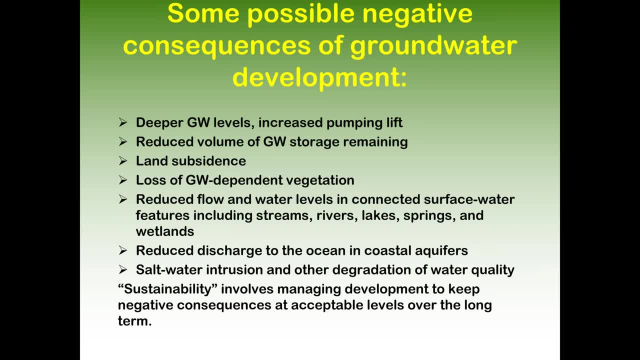 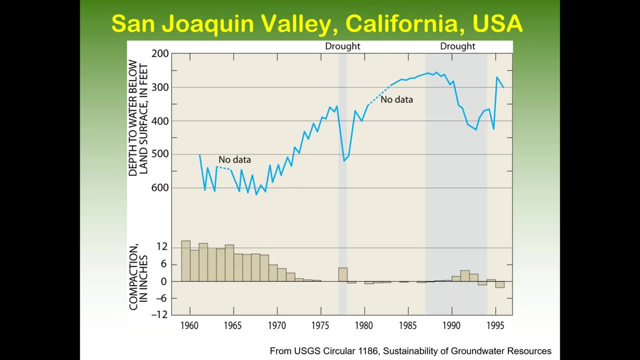 acceptable levels over the long term. And again that kind of involves society as a whole and not just the scientific aspects of it. Here's an example of groundwater use In the San Joaquin Valley in California, which is a very large percent of certain crops. 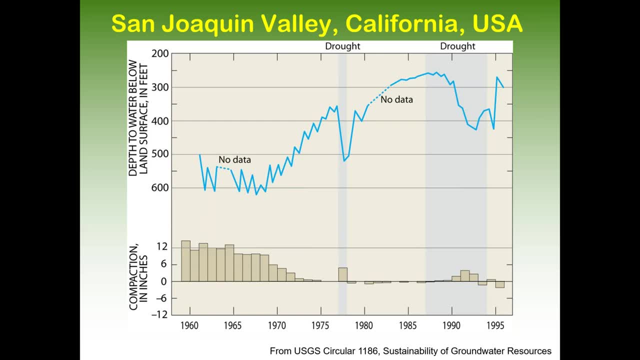 in the United States are grown there And originally it was irrigated with groundwater. This graph starts around 1960.. And you see we're getting at that point. depth of water is almost 600 feet, So the pumping had really drawn down the water And, as a result of that, in that bottom 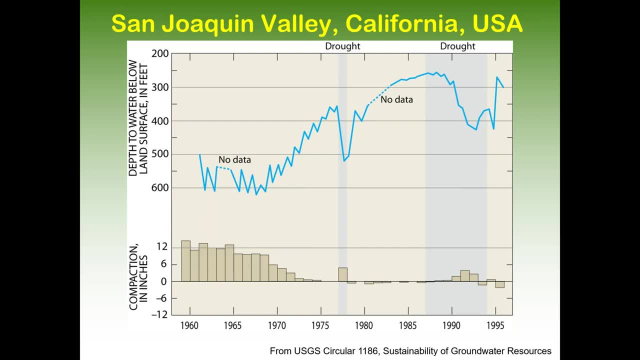 graph we're showing compaction in inches And that's yearly numbers. So eventually, maybe by the early 70s, surface water was brought in because we had one place in the Central Valley Where I think it was pretty close to they had pretty close to 30 feet of land subsidence. 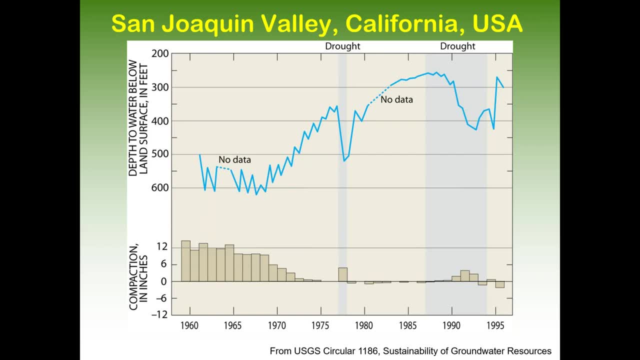 But, as you can see, the water levels are coming up, starting at about 1970. But then we have this drought in the late 70s and water levels immediately go back down by Perhaps 150 feet, And associated with that there was some additional land subsidence. 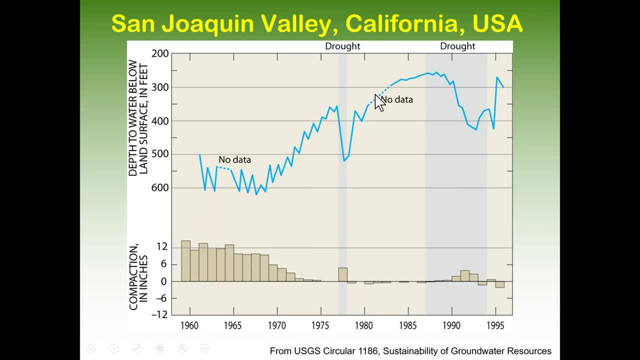 But then when surface water again becomes available, then there's a recovery, Another drought period around late 1980s, And then water level declines. And then we have a drought period in 1980s, And then we have a recovery, Another drought period around late 1980s, And 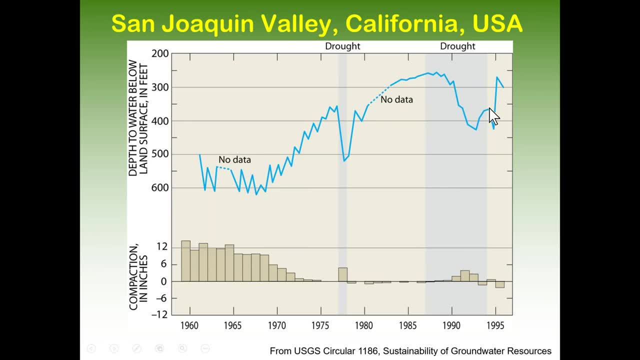 then water level declines And then we have a drought period in 1980s And then water level declines, Some additional land subsidence or compaction And then finally a recovery. But anyway, this is an example of using groundwater to kind of get through droughts. But there 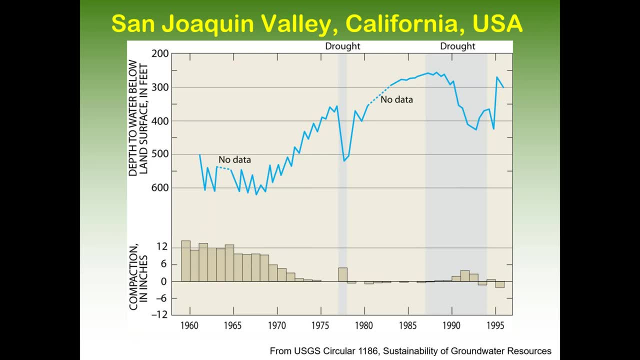 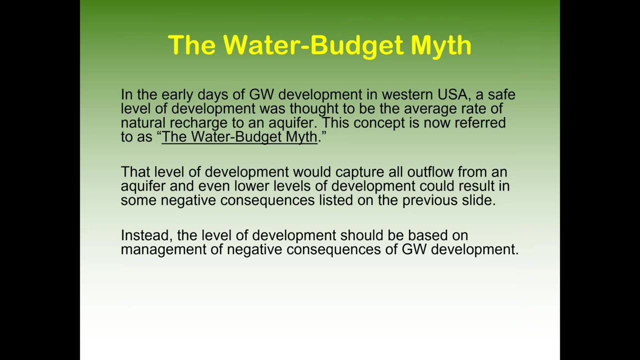 is some negative consequences associated with it, But maybe that's tolerable to help get through these periods. Okay, Thank you Mark. Thanks Mark. Thank you Mark. Thank you Mark. Now there's something that we call the water budget myth, and I recall that when we talked 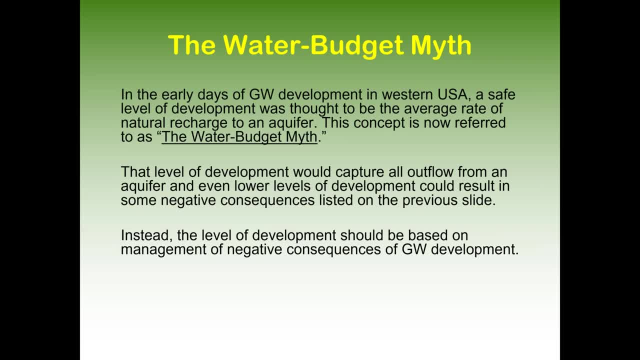 about safe yield. we say it's often set to the amount of recharge that occurs in an aquifer, But we now say that concept is the water budget myth that the safe level of development is the amount of recharge, Because there could be a lot of negative consequences even at levels that are much lower than that. 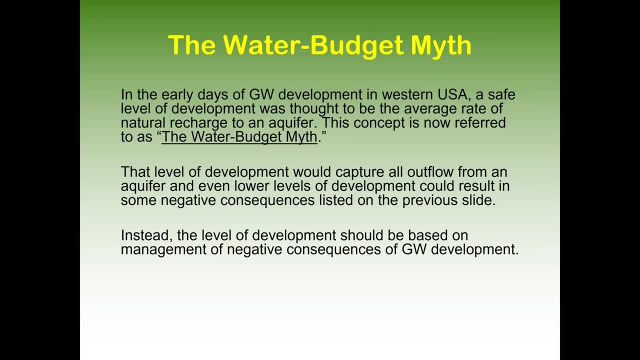 And instead of looking at how much water is being recharged, we need to look at how the effects of that development and the original concept by Bridenhoff and his colleagues of the water budget myth was that you should look at how much of the 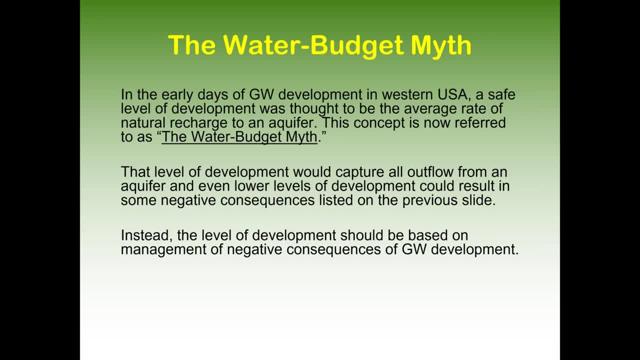 outflow that could be acceptably captured. So if you have groundwater flowing into the aquifer and then discharging to some streams and wetlands and things like that, the effect of the pumping- and I'll be going into this more later- is going to be how much. 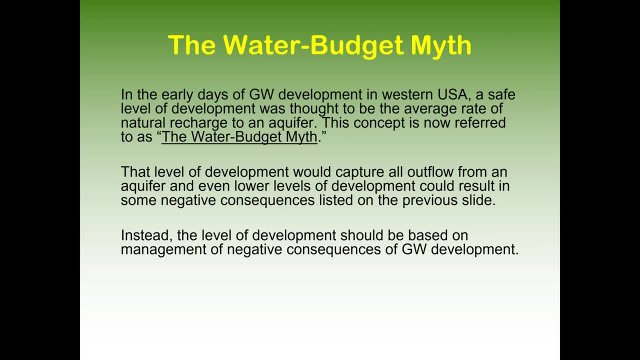 of that outflow you can capture? I mean, would it be acceptable to dry up the streams and the evapotranspiration areas? That is one of the consequences, But there could be other consequences too, like land subsidence and drying up existing 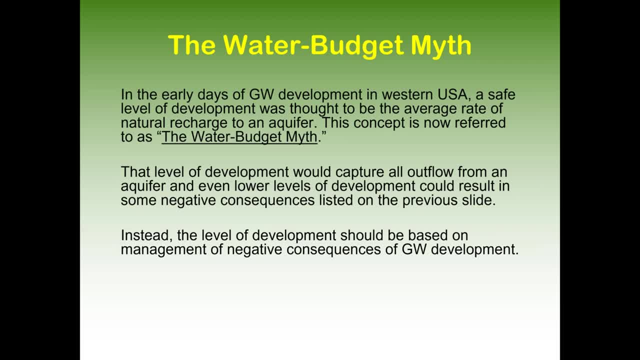 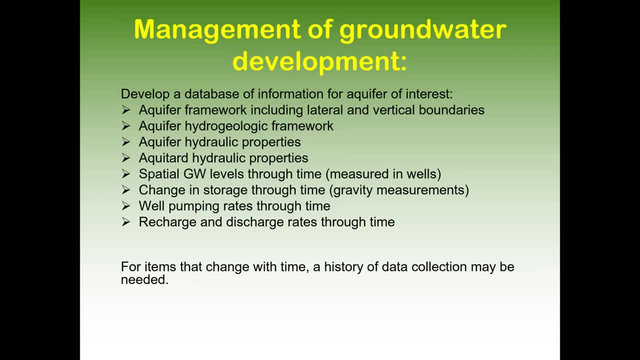 wells and things like that. So to manage groundwater development. I'm sure Mark has been talking to you a lot about this, But I don't think you can do that. But the way that we're looking at it is is that there needs to be a way to manage that. 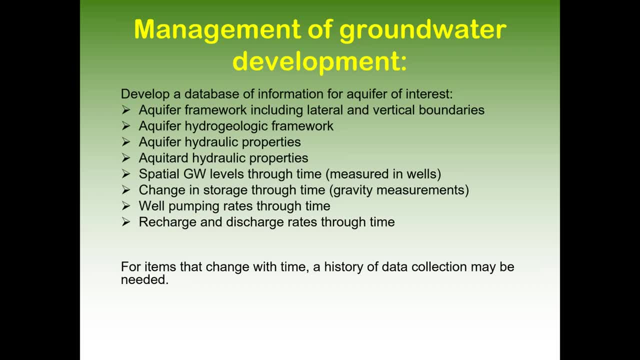 in the sense that we were talking about before. So, in the case of the water flow, we're developing a database and all this is going to be leading up to developing a numerical model that can be used in the management. But so you need to know the aquifer framework, the lateral and vertical boundaries and 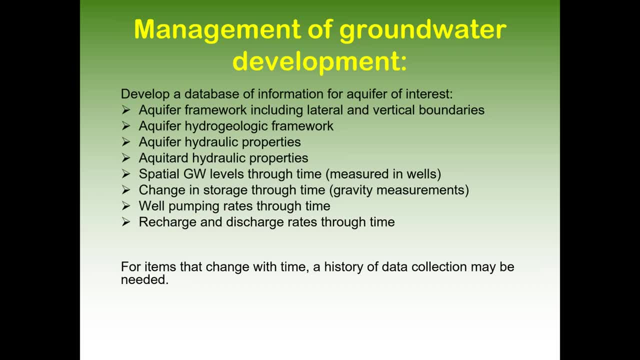 what we would call the aquifer hydrogeologic framework, kind of clay layers you have. is it a multiple system where you have connected aquifers and then the actual hydraulic properties, like the transmissivity, hydraulic conductivity, storage coefficient of the aquifer and also of 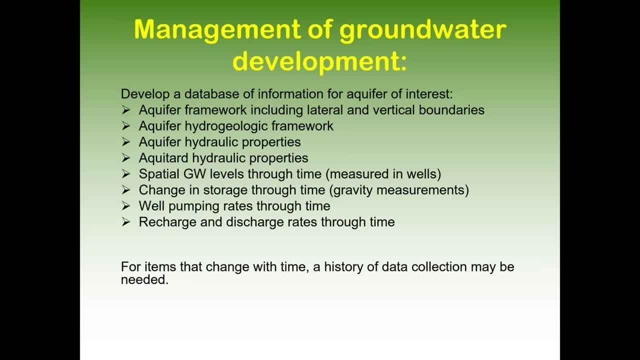 what we call aquitards, which are the low permeability layers like clay and silt that are embedded in the aquifer, and then groundwater levels measured in wells. and that's something that has to be done continually over time. change in storage through time. we we do that with gravity measurements and then some rates. 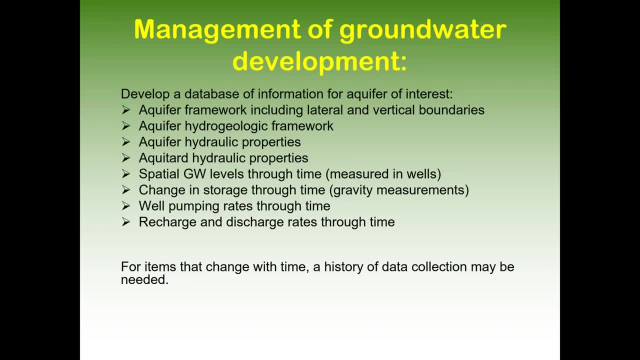 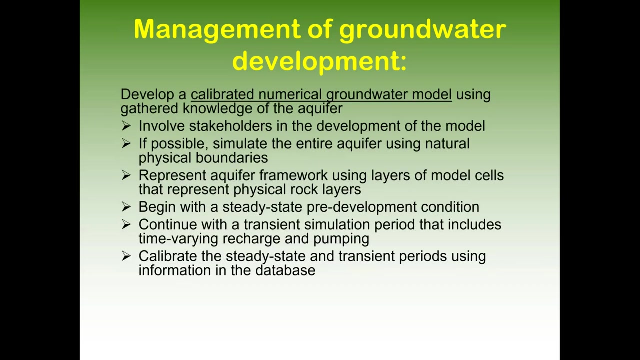 of in the flow and outflow to the aquifer, including how much Wells pump through time and then recharge and discharge rates through time. so for these temporal data sets a really long history is good, so the sooner you get started with that, the better it is. and then, assuming that you do have enough data you have, you develop a. 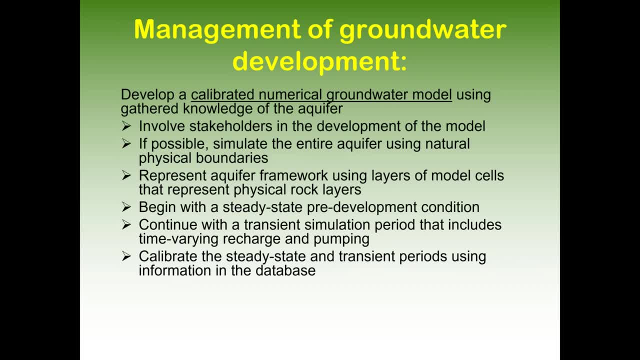 calibrated numerical groundwater model using this information. it's always good to involve stakeholders in the development of the model, so if you have farmers or groups or municipalities that use the water, have them be a part of it. you know, update them on what's going on. you'd represent the aquifer framework using layers of modeled cells that would represent 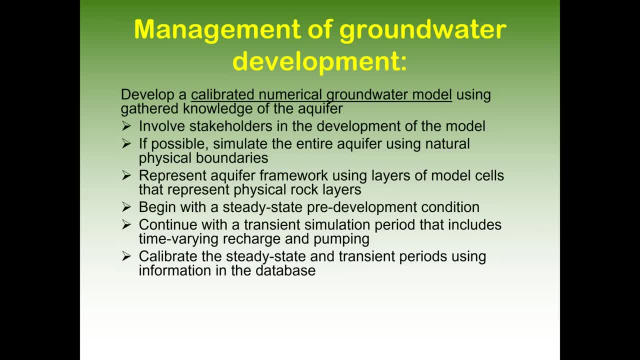 physical rock layers and then begin the model with the steady state pre-development condition using long-term average recharge, and that would result in kind of a a good starting point. and then you'd have what we call a transient simulation period. that could include time varying, recharge and pumping, and then 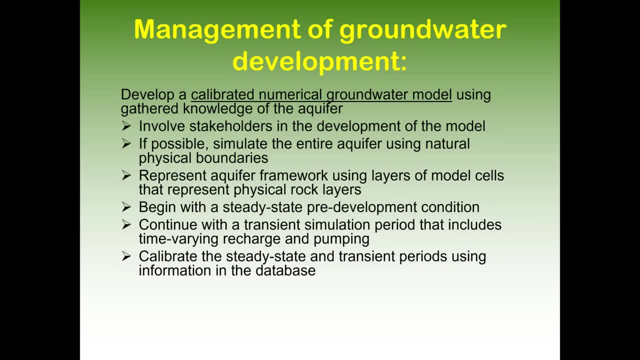 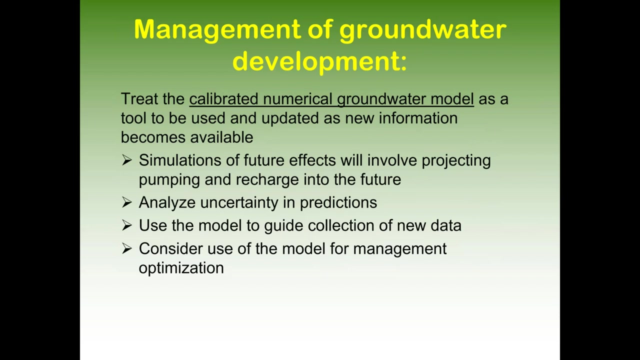 um, you calibrate the steady state and transient period using things like water levels from Wells and the database, and if you have any observe flows like how much groundwater discharges to streams, that would be important calibration information as well. um, and then you kind of treat this model as sort of a living tool that's used and updated. 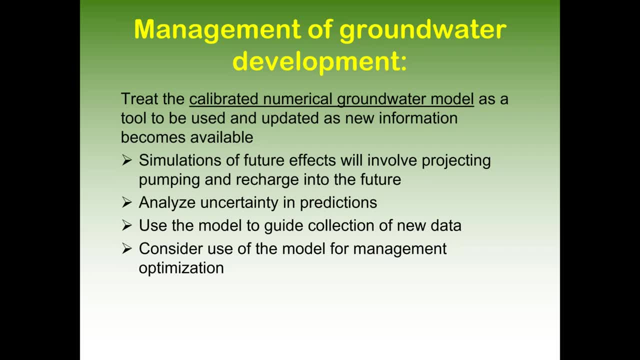 as new becomes available. it's always difficult when you're projecting into the future to know exactly what to put in for pumping and recharge, how that's going to vary in the future, but you can sometimes make assumptions and see what the effect would be. if possible, it's good to analyze the uncertainty and the predictions and then 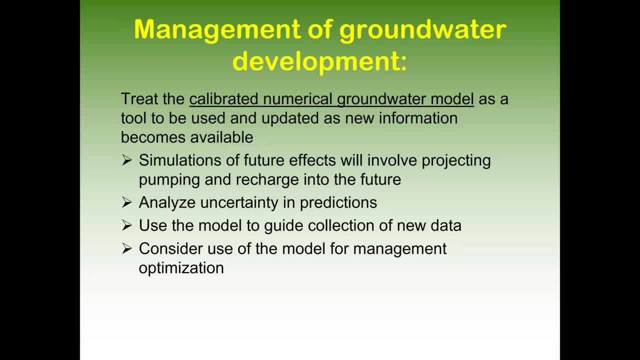 you can use this model to help guide a new data collection based on where, if you had data in certain areas, would it improve the model or not. there's ways of doing that and then, if it's a really good model, you can do something called management optimization and try and answer questions. like you know, where is the optimal? 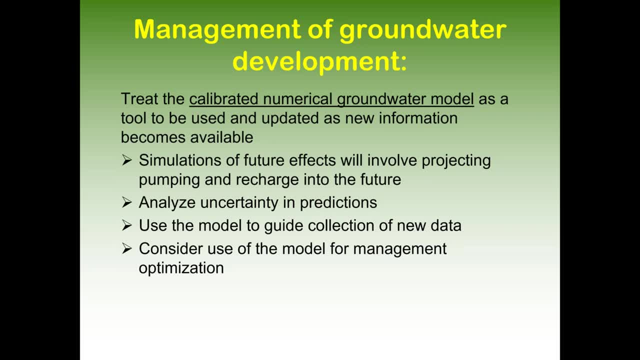 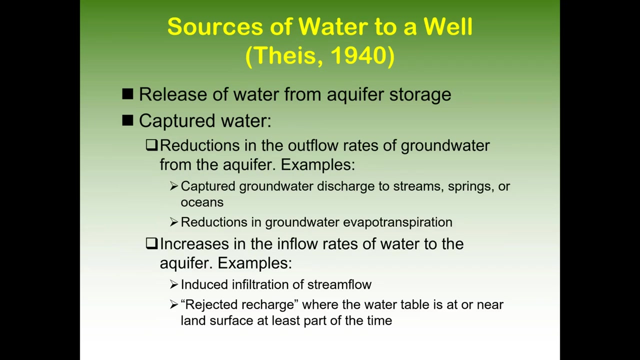 location for a new well or optimal pumping rate, and you can also. I've not got into water quality and contamination and things like that, but a good model would be a start for those kind of analyses as well. okay, I'm going to switch now to sources of. 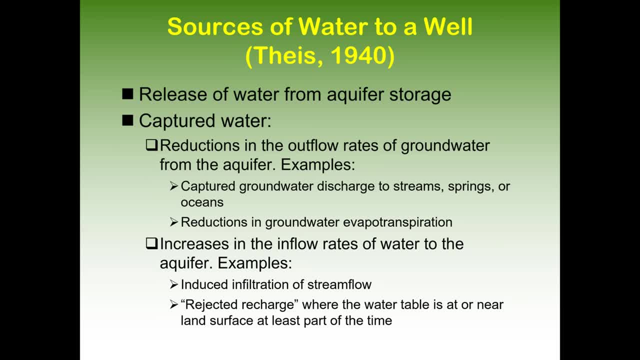 water to a well, which is related to this, to kind of understand what happens when you pump a well. so any groundwater hydrologist will know the name tise because, uh, he made the equation that we used to analyze aquifer tests. but he also observed, uh, in a 1940 paper, that when you pump a well, 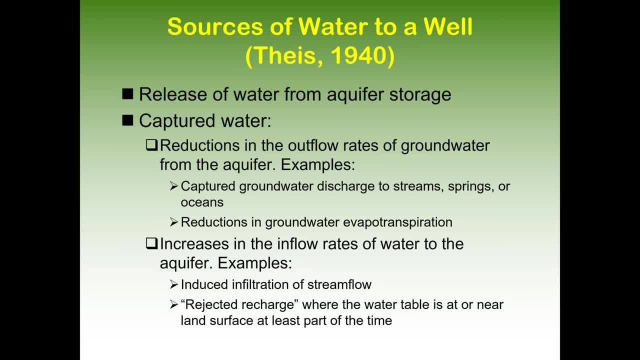 initially all the water comes from arc for storage and then with time the cone of depression spreads out to where there's discharge from the arc for, for example, like groundwater flowing to streams and rivers, and that dry down reduces that outflow and then it can also increase inflow rates by. it can actually make, if you. 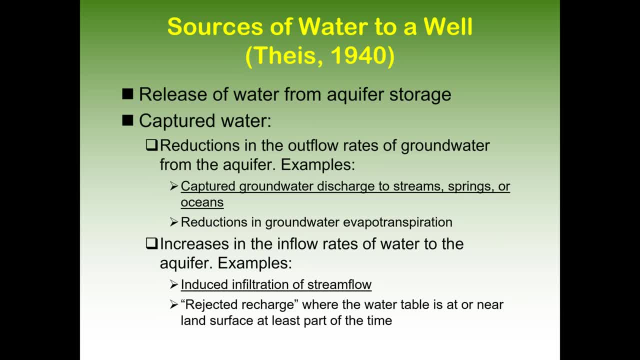 have a place where the stream is losing water to the aquifers, it can increase that loss. so actually the pumping is causing more water to flow into the aquifer. and then there's another concept where, if the water table is right at the land surface, pumping a well creates some space for recharge to occur. that wasn't. 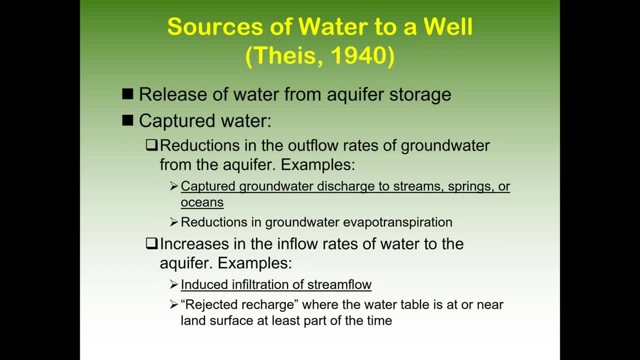 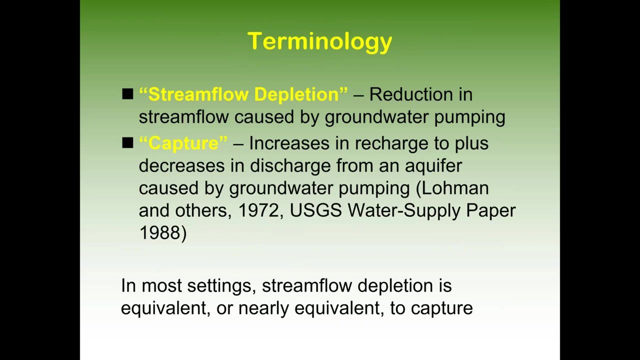 there before. so we recall that capture of rejected recharge- and I'll say that most capture- is going to be reduced. reduction of groundwater outflow from the aquifer and that's going to affect the amount of streamflow. all right, so streamflow to please share is reduction in streamflow caused by groundwater. 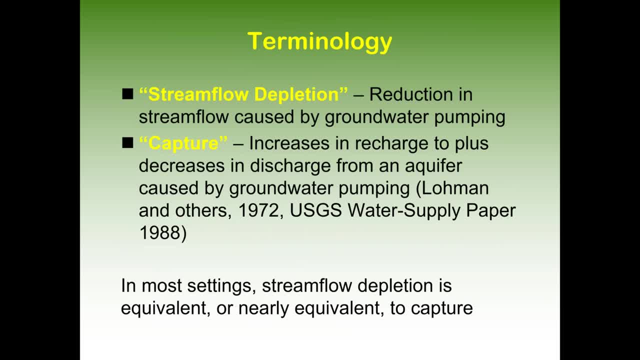 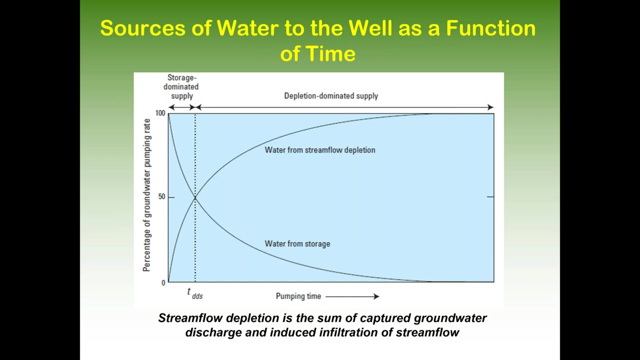 pumping and capture, increase in recharge plus decrease in discharge, as I said in the previous slide from using Tice's observations. So in most cases streamflow depletion is equivalent or nearly equivalent to capture, And the way we represent this graphically is I sure wish I could find the. I'll just 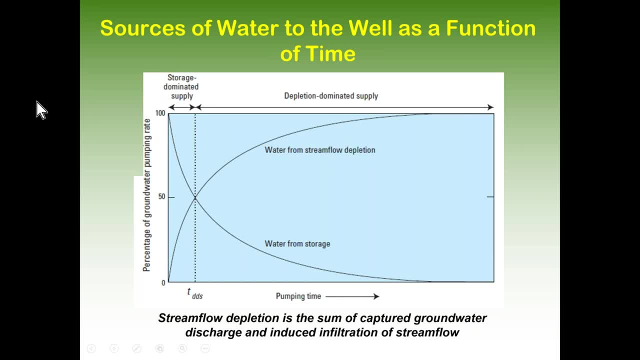 try. No, but I don't think you should watch that because you are busy. You're not that busy, So you'll tell them that I was busy. No, but I think it's you're saying. you should understand when I say I was busy. how? 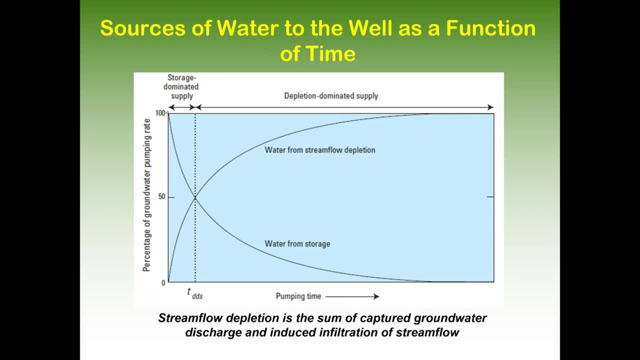 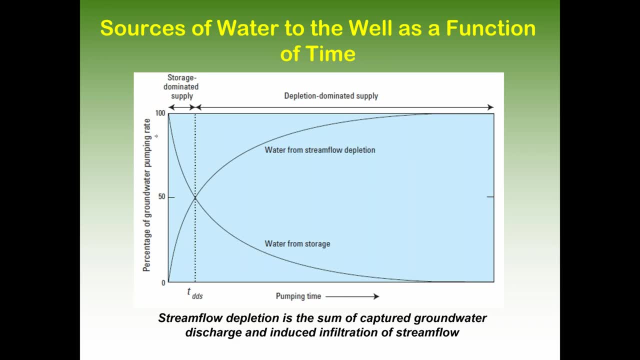 So please carry on. Okay, All right, Maybe you can see this arrow I have now. So what's the question? When you first start pumping a well, this curve up here says that 100% of the water is coming from storage in the aquifer. 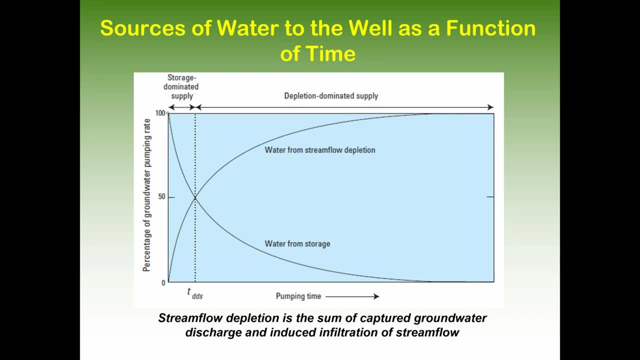 And that's either draining of pore spaces or it could be elastic storage in the aquifer, where water expands and the sediments contract or compress, But with time, As that cone of depression moves out, say to streams and rivers. maybe you have this. 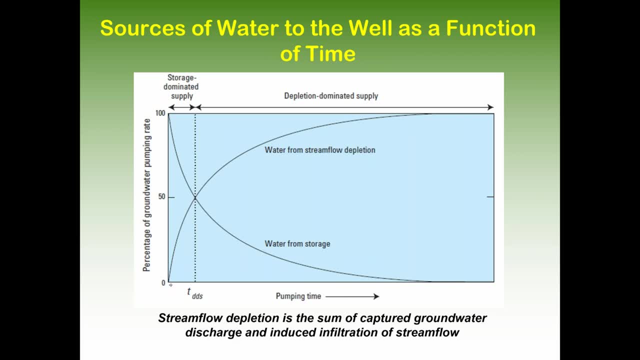 capture or streamflow depletion, which initially none of the water is coming from that. But if you pump long enough, all of the water is going to be coming from streamflow depletion or capture And none of it from storage. This is what we call a new steady state condition. 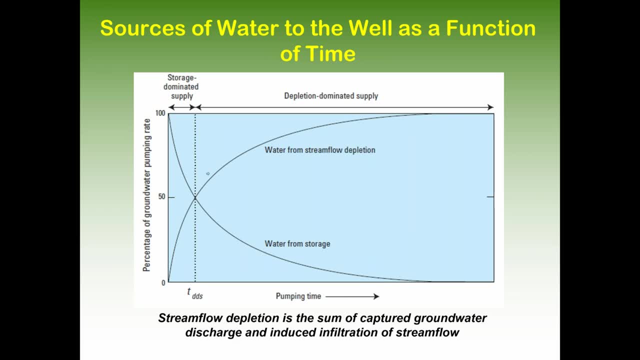 And then we've marked these two curves where they cross. It's kind of a point where on one side you have storage dominated supply- More than half the water is coming from storage, And on the other side we have depletion dominated supply, Where more than half the water is coming from depletion. 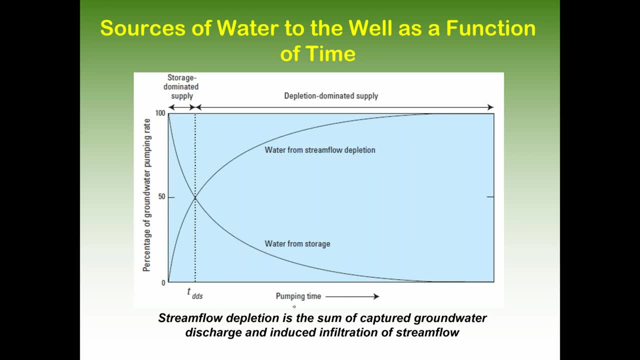 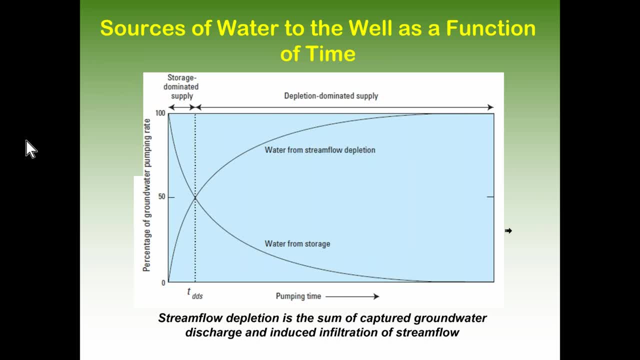 Let's see, Let's see. Okay, Let's see. It's not going. Page up and page down is not working. Can you use the new line button to see if it works? It's working. A new line, Let's see. 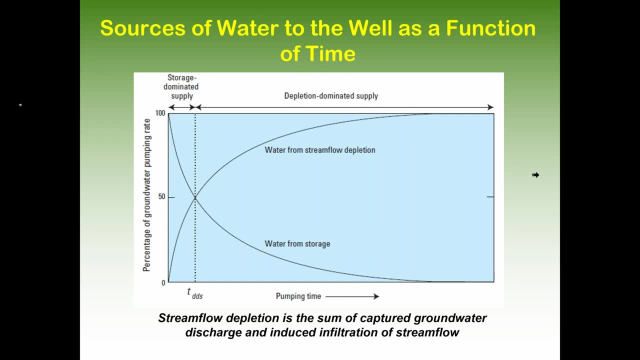 Okay, see my pause. I might have something to do with the pointer. I'm sorry. what were you saying that it might have something to do? did you use a pointer from the gotowebinar tool or is that your? yeah, I use the arrow from. maybe you from the? 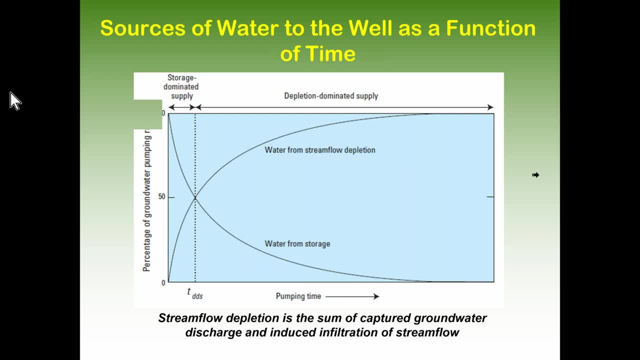 little side side panel. okay, so maybe there's a, maybe there's a lot that error, and then see if it works again. and might, or it might be that because you have that arrow, it overrides your computer's ability to go up and down. here we go. yeah, I'm drawing mode, let me do that. huh, well, I went to non drawing mode. 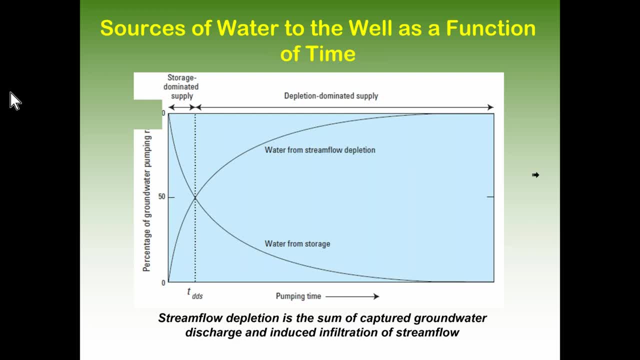 let me see if I can. okay, now I got it back. yeah, okay, so I'm back. so this is our graphical representation, and it might be more complicated than this. I'm showing the next slide. when you start pumping the well, all the waters coming from, stories change, but the cone of depression may enter into a vapid. 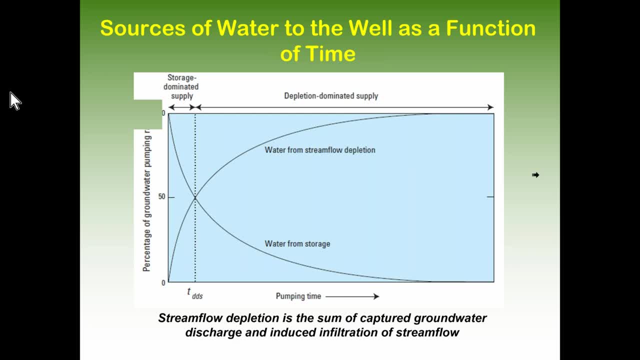 transpiration areas where you have plants that use groundwater and it could reduce the amount of water that those plants are using by lowering the water table and then it could deplete stream flow and then, as a cone of depression, that's going to slow down Syndromere at the lowest concentrations in that. 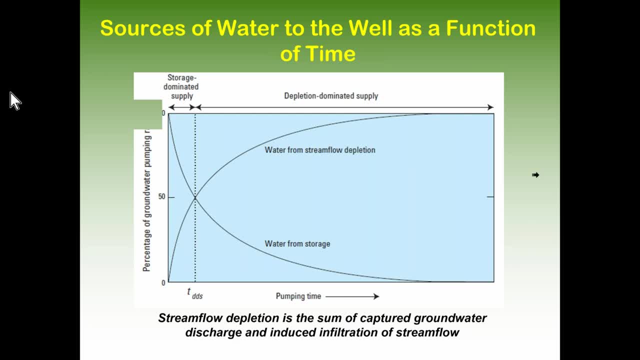 crystal-co气 curve if we are flowing water out to the bottom and we change the temperature of the water in a provincial tank. well, that today I just thought would be an interesting idea, and that's one example of an example of moving a vessel everyday and not picking up the water while it's at the 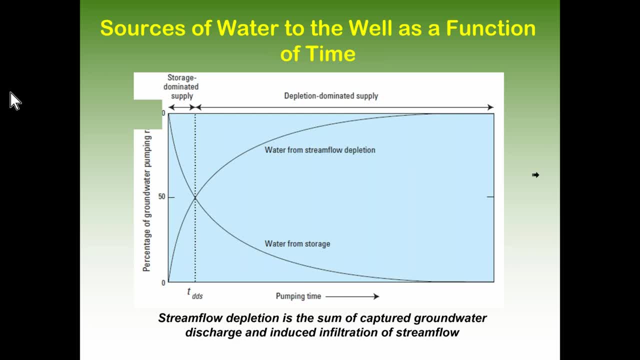 surface of this waterbereich in that room. so what this jadi opportunities for, It's either going to be storage change or total capture. So this is, as I said, a really important issue in the United States. Here in the semi-arid southwest, I would think that this – we have – this is where this 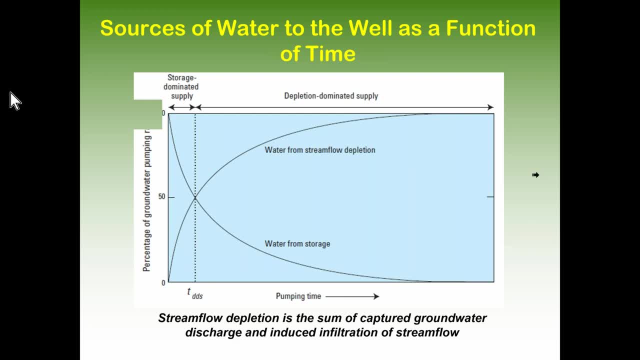 issue occurs, but actually it's a big problem. even in eastern USA, Groundwater pumping is capturing water that would otherwise go to streams, So even in more humid areas, people are very concerned about this and they want to protect the remaining. 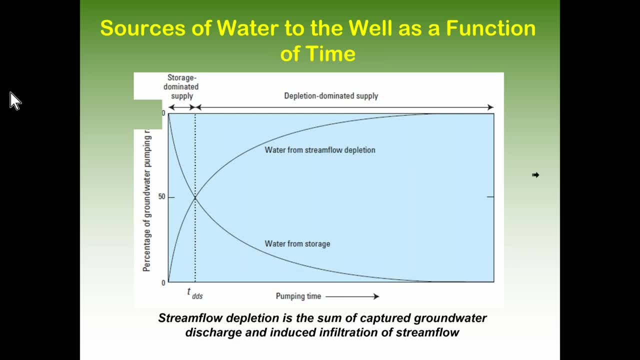 They want to protect the remaining riparian ecosystems, And then also the holders of existing surface water rights. they don't want their flows reduced. So this is kind of a way that people can take water from streams without really having a water right. 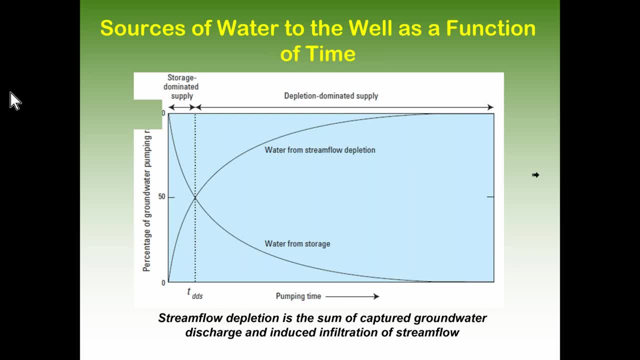 In a lot of cases, the groundwater laws are not sophisticated enough to recognize that pumping a well can take stream flow, So you – yeah, go ahead, I'm going to go back to the source of water to well slide. Okay, So if there is – 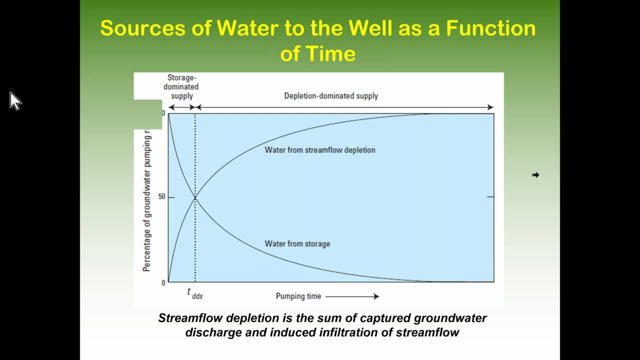 Sources of water to a well. Yeah, So we are stuck with that one, which is the one that caused the problem. Yeah, I don't know if you can maybe stop the presentation and restart and then just go straight to that page or – because it's not showing what you are seeing on your computer clearly. 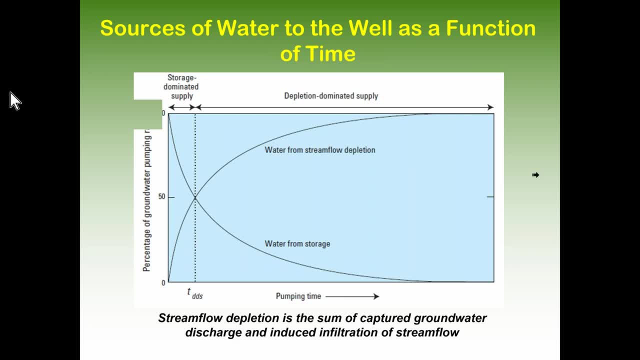 You're talking to a slide that we're not seeing. Yeah, Yeah, So I'm going to go back to the source of water to well slide, Okay So – yeah, So I'm going to go back to the source of water to a slide that we –. 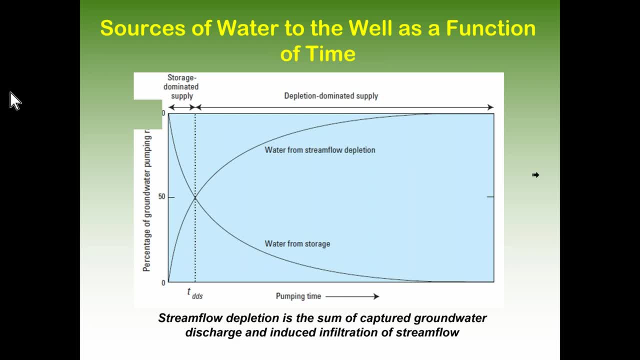 All right, Oh, it says show screen is paused. Okay, Freeze on last screen. Now. it says it's showing my screen. now Let me see if – Yeah, Yeah, Okay, So it's showing my screen. now Let me see if I can –. 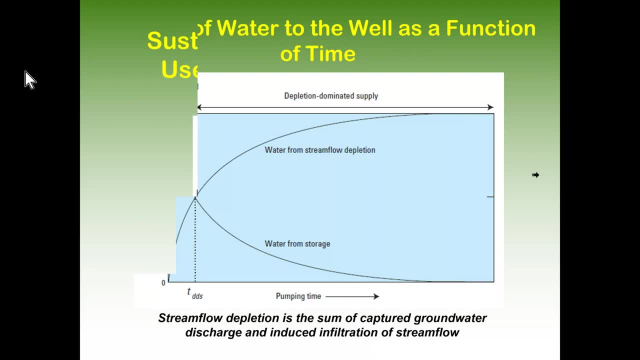 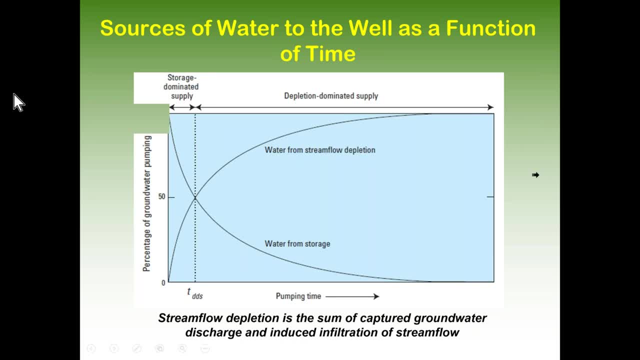 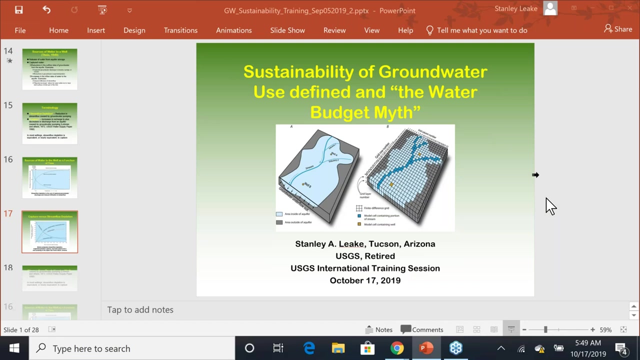 Okay, But now it's not going forward. Oh Wow, It's –. It is still on the – Yeah, Yeah, Yeah, on that same slide. so i don't know if it's more worthwhile to close the presentation and restart it and just go straight to the. okay, i could do that. i mean that that's easier. thank you, all right. 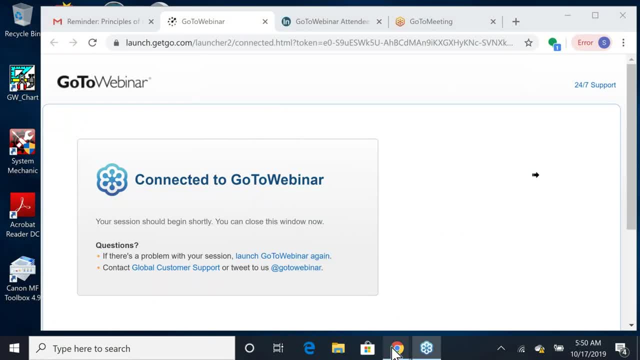 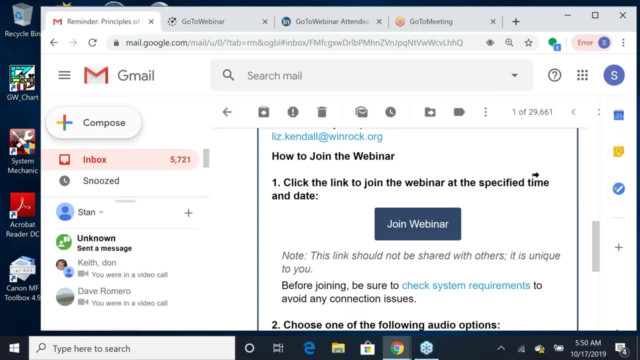 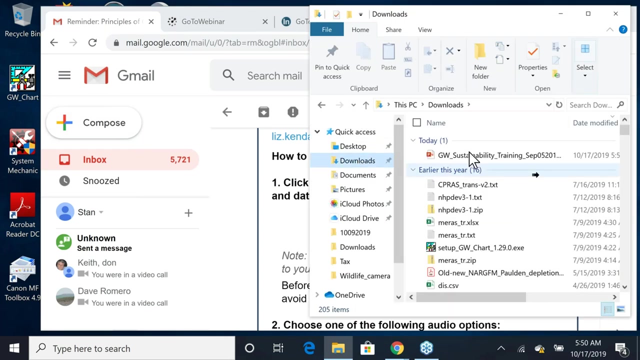 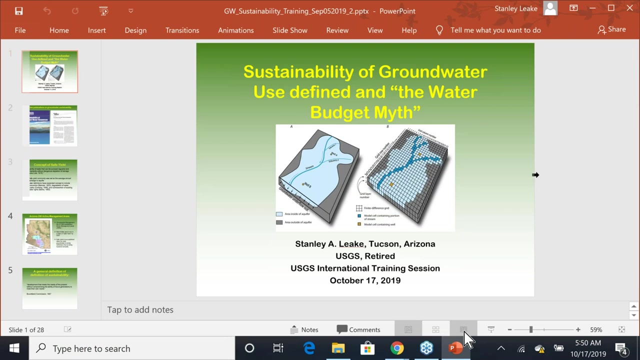 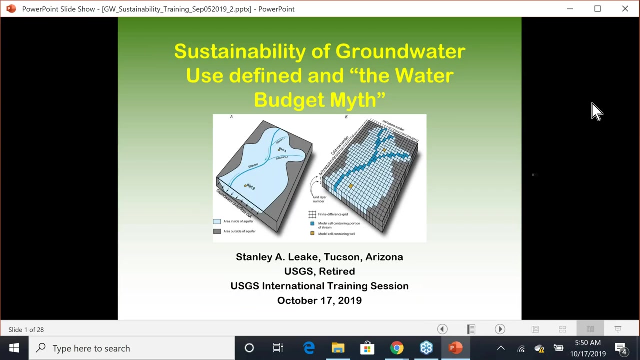 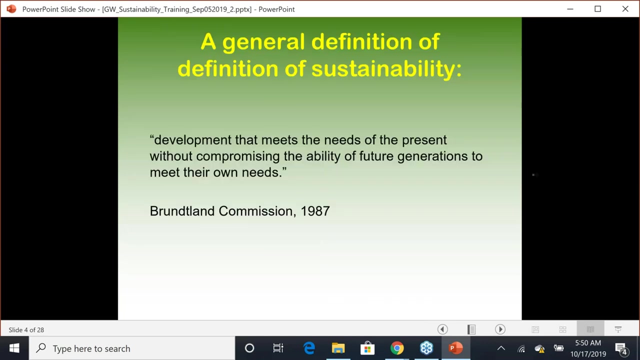 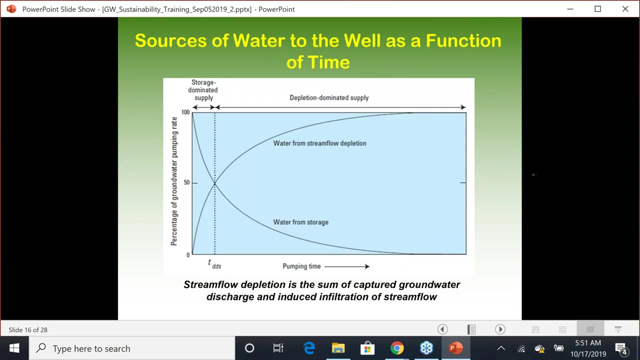 all right, oh, all right. well, okay, i guess i won't try that arrow anymore. that seems to cause a problem. are you seeing the um? we're seeing the presentation again. yeah, and now you're moving for the slides. thank you, yeah, this is where we were stuck. that's where we're stuck. 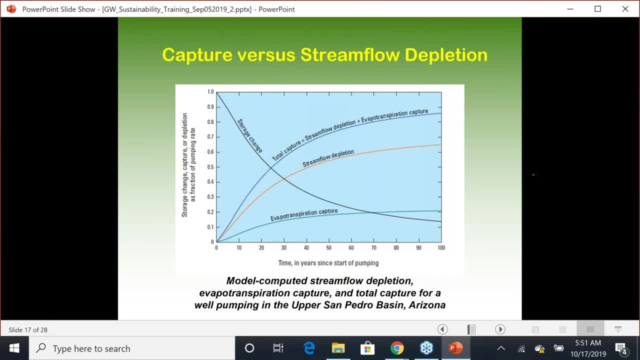 all right, all right, and i think i described this one, but you didn't see it. um, i was saying you could have multiple places where water could be captured, from evapotranspiration or streamflow depletion, and then the total capture would be the sum of those two and this. 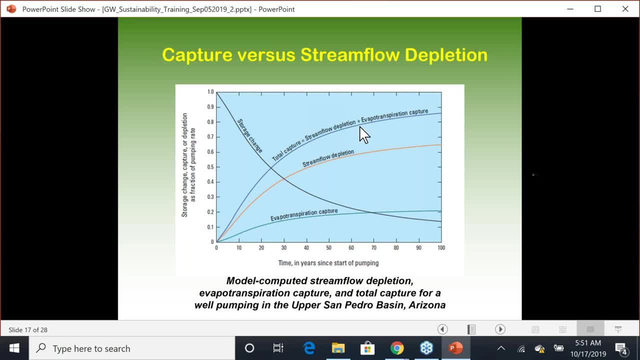 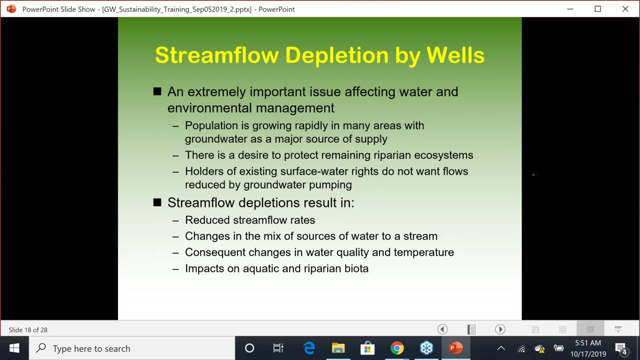 total capture plus the storage. storage would be the sum of those two. change are always equal to the world pumping rate. so those were kind of the points there then I was discussing that this is an important issue, not only here in this semi-arid southwestern US, but even in the more humid areas people are 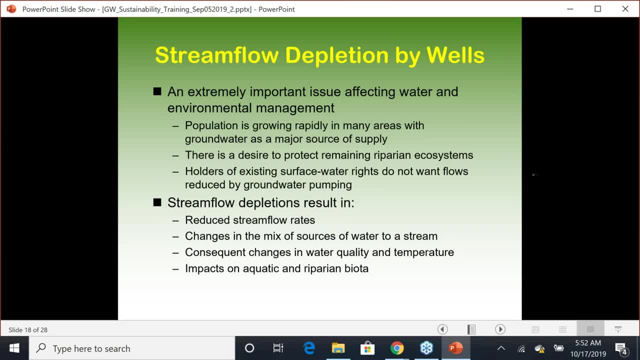 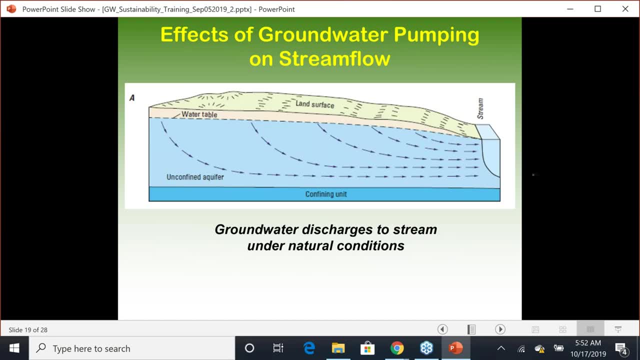 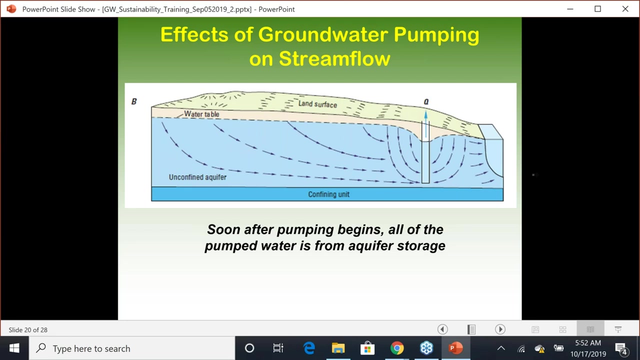 very concerned about this issue. so the kind of progression graphically is that without a well pumping you would have recharge to the aquifer, to the water table and then water discharges to the stream. excuse me, at some point, if you introduce a well, you lower the water table, you take water from storage, but you may still have the 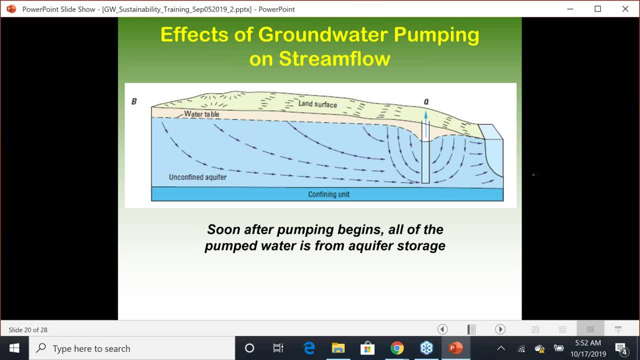 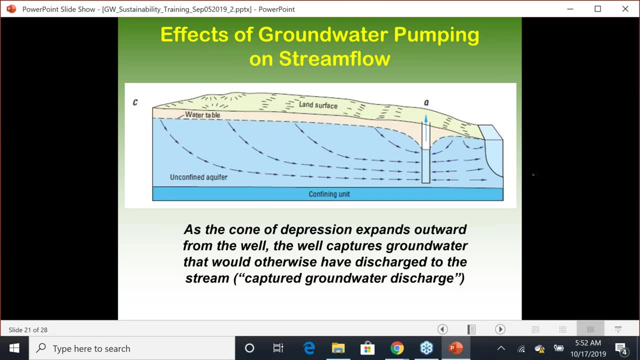 same amount of water discharging to the stream because the Kona depression hasn't reached the stream yet, and then at some point you may reduce that gradient to the stream as the Kona depression goes out. so you have captured groundwater discharge to the stream. um, but you, you may still have some discharge to the stream, just not as much. 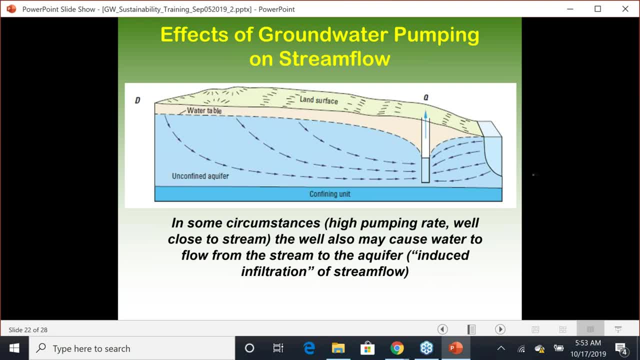 and then, um, if you have really high pumping rates or the well is very close to the stream, it's possible to reverse that gradient to where now you're actually drawing water from the stream. um, and this is a more extreme case, with what we call induced infiltration of stream flow. 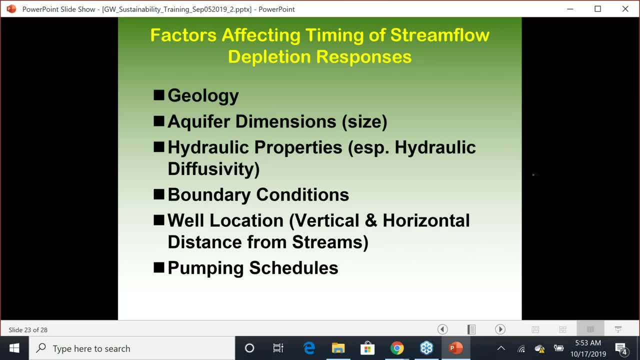 uh, the factors that affect the timing are the geology, the aquifer dimensions, the size of the aquifer, hydraulic properties like diffusivity, which is transmissivity divided by the storage coefficient, the boundary conditions where you might have no flow boundaries, or other things that affect the change in head. 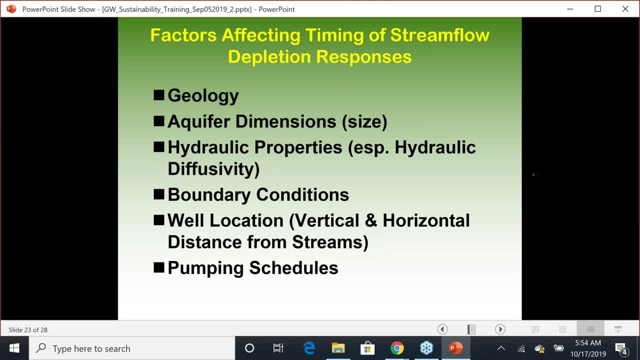 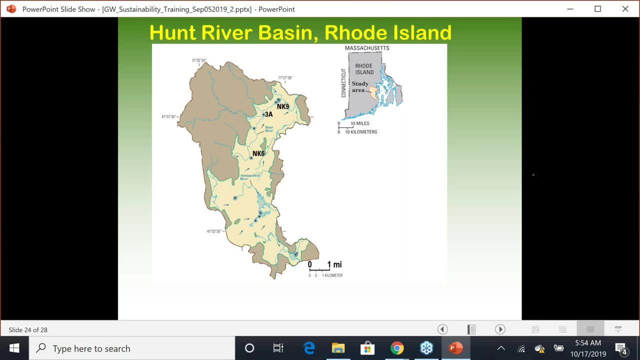 a well location, the how far it is from the stream, both vertical and horizontally, and the pumping schedules, how often you pump and that sort of thing. uh, to show you, um, some differences in timing, This is in our smallest state, Rhode Island, a very small basin called the Hunt River Basin. 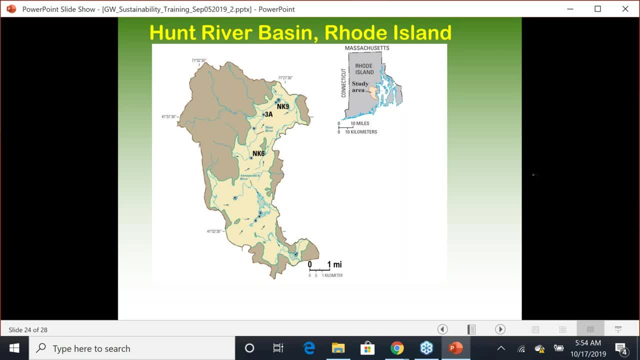 And it's just a handful of miles wide and maybe- I don't know- 10 or 15 miles long, And there's a few wells that we have shown here, And this is the streamflow depletion calculated by a groundwater model for these three wells: 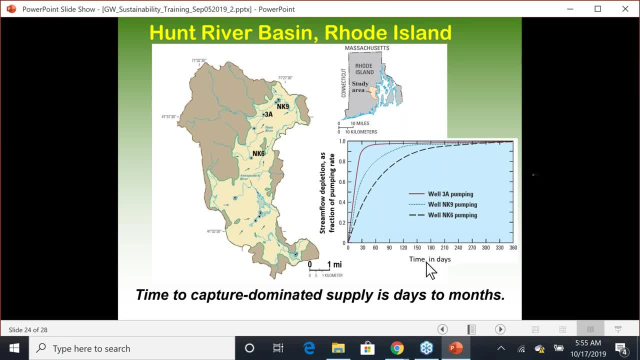 And notice that the time on this graph is measured in days. like the whole graph covers about a year, So within about a year if you pump any of these wells, essentially all the water being pumped is coming from streamflow depletion, So it reaches this new steady state condition fairly rapidly. 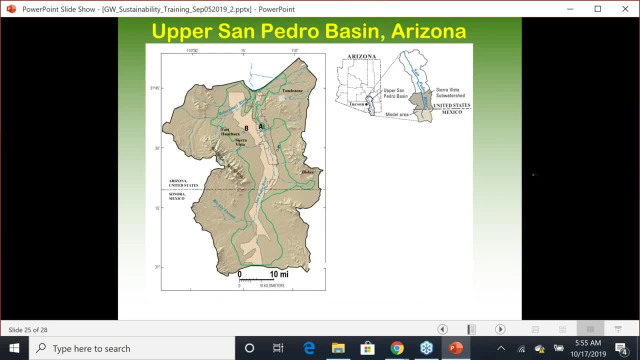 Now contrast that with out here in the Southwestern USA we have this basin that kind of starts in Mexico, flows to the north into the USA. This also with the groundwater model. we have these two hypothetical well locations. One is actually fairly close to the river. 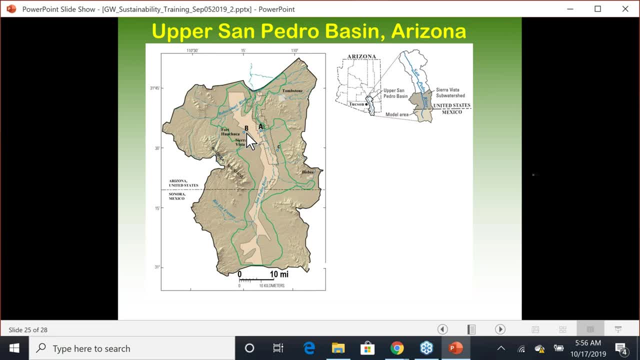 And one is maybe about six or seven miles away, And here we measure time kind of more on the decadal scale. So it's a very different schedule And we like this well. B, which is further away, If it pumped for 100 years. 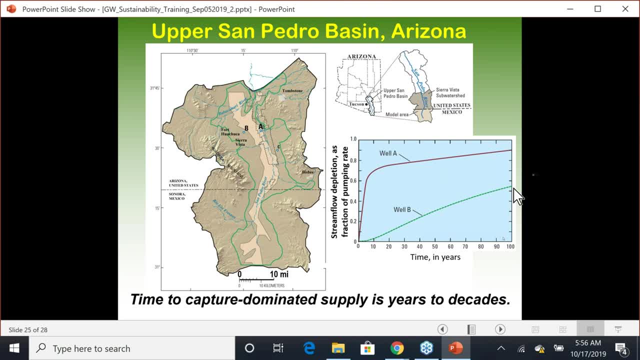 you would just barely get half of the pumped water coming from capture of surface water. And even well A, which is fairly close, probably within a mile or two of the stream- it's still very close- doesn't reach a steady state in this hundred year period. so there's a big 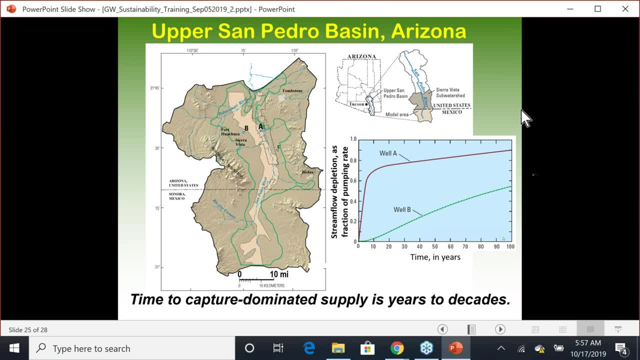 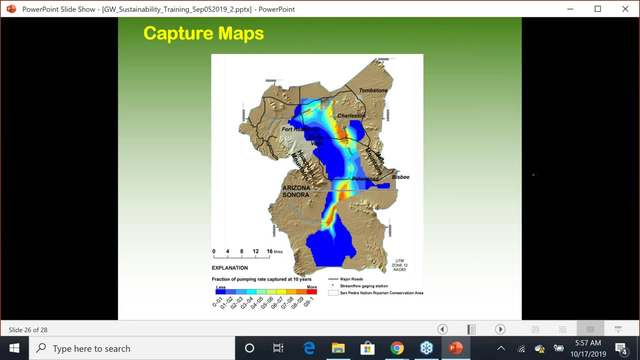 difference, especially the size and the distance from the pumping wall to the stream, control the timing of that capture of surface water. one thing we've done is made something we call a capture map. this is for the San Pedro Basin and what this particular one says, that if you pumped a well for ten years, this 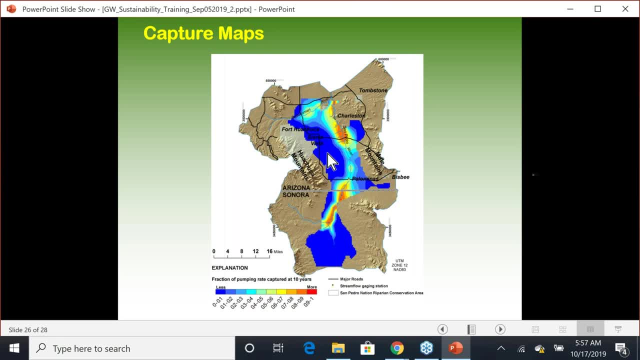 would give you the percentage of the well pumping that would be coming from captured surface water. so if you were in this dark blue area and you pump for ten years, less than 10% of the water would be coming from captured surface water. and if you pumped for in this orange area, for example, it might be more like 70 to 80%. 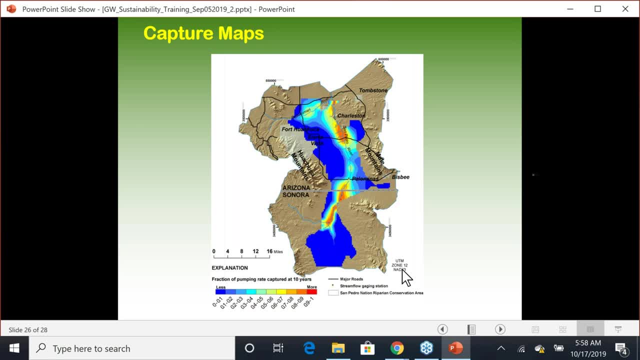 of the water would be coming from captured surface water socket. this has been a valuable tool for people to use to understand the timing of timing capture and I'll just say that in this particular basin it's kind of one of the last remaining desert streams. it doesn't have any dams on it and it's got. 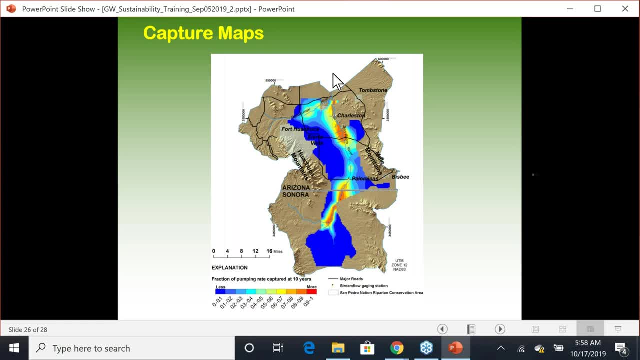 a riparian trees by the river. that's good habitat for birds. it's kind of a internationally known birding area, and so the people that live here in the town of Sierra Vista, I think for the most part- want to see this river preserved. they don't want to see it dried up because of groundwater pumping. so this 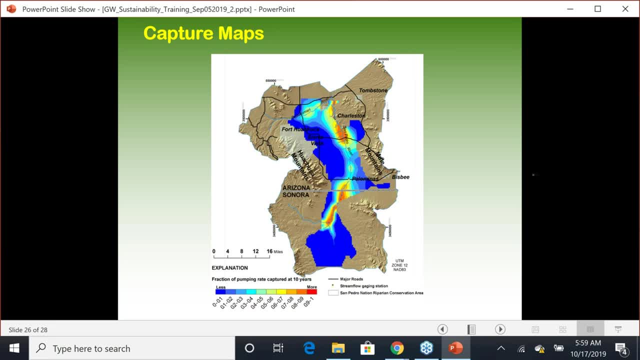 is kind of what I was referring to earlier is maybe a societal effect of people deciding what's important for their area. so, on the other hand, groundwater is their only source of water in this space and they don't have any reliable surface water supplies, so they're doing all they. 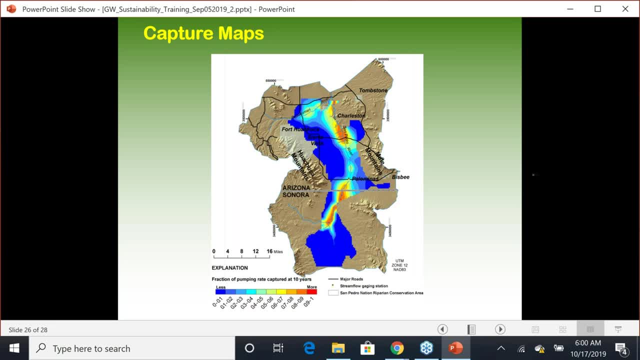 can to reduce the amount of water they use and to make use of the water that they use, and to make use of the water that they use and to make use of water that returns that's not consumptively used in their houses and businesses, and things like that. so that's very important. it's a good 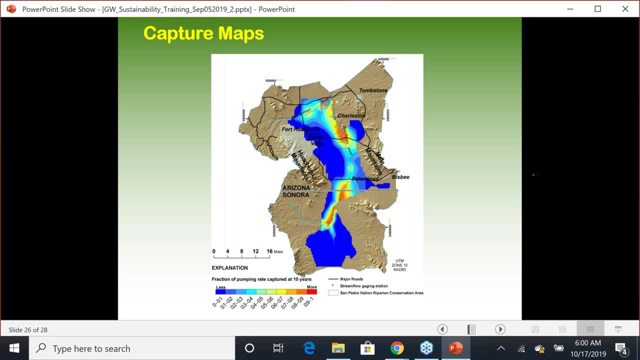 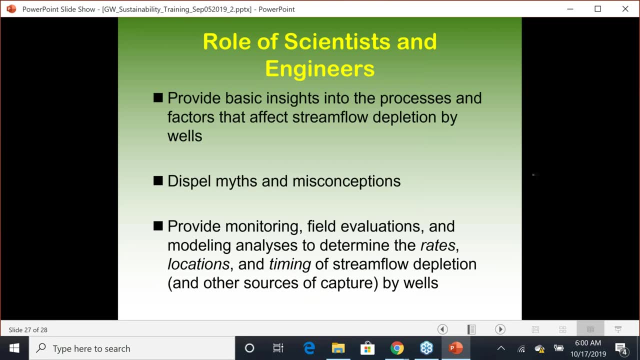 example of kind of people caring about their. their resources are related to groundwater, so the scientists and engineers, we can kind of make our models and tell you what factors are important that might affect streamflow in any given area, dispel myths and conceptions that people might have about groundwater pumping, provide 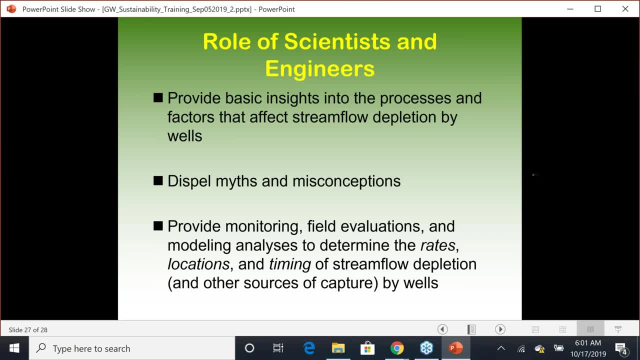 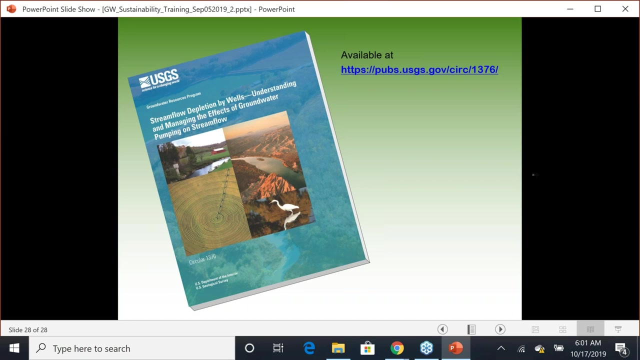 monitoring, field studies and modeling to determine the rates and locations and timing of capture by groundwater pumping. and I guess this is my last slide right here. if you are interested in this topic of streamflow depletion by Wells, we have this circular 1376 which again you could find on the internet since they all USGS publications. 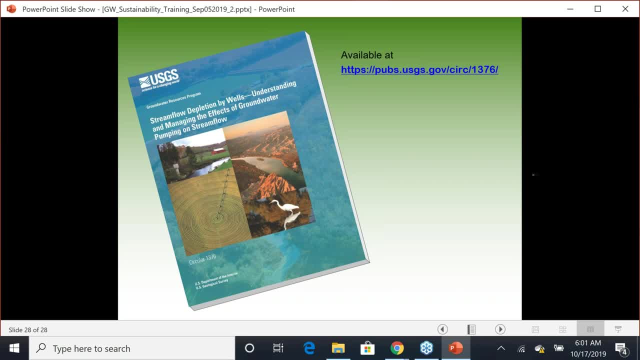 which, again, you could find on the internet, since they all USGS publications are are online. so this kind of covers this topic in a lot more detail. so that's essentially what I had for you this morning. I don't know, do we have. that's essentially what I had for you this morning, I don't know. do we have? 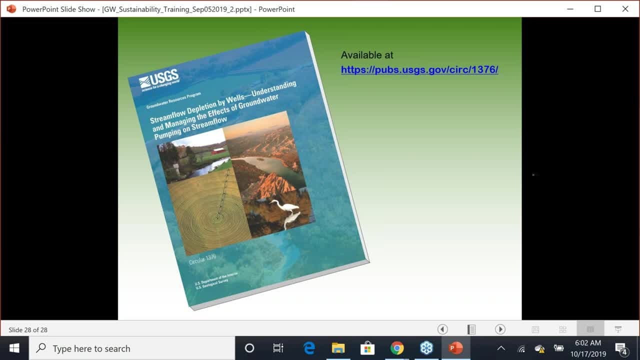 time for questions or discussions. yes, thank you, Stan, we do, but before I open the floor for questions and discussions, I would like to give the word to mark from USGS is basically our connection between the big data analytics and transponder, a water management, collaboration with Southern Africa and 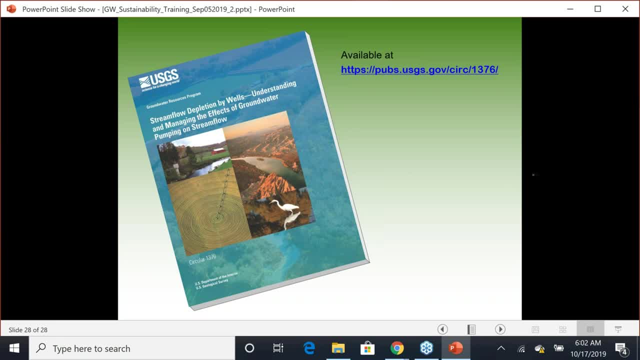 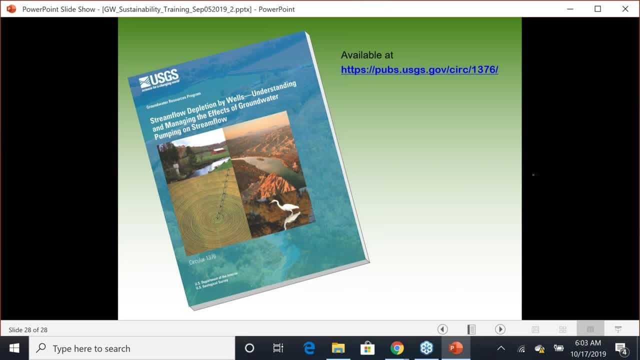 Mark, Mark, I wonder if I could send him a message. I was actually thinking the same let's. let's carry on. yeah, okay, I guess we could open it up to anyone else then. yes, before we open up to the floor, I just wanted to say thank you to you for. 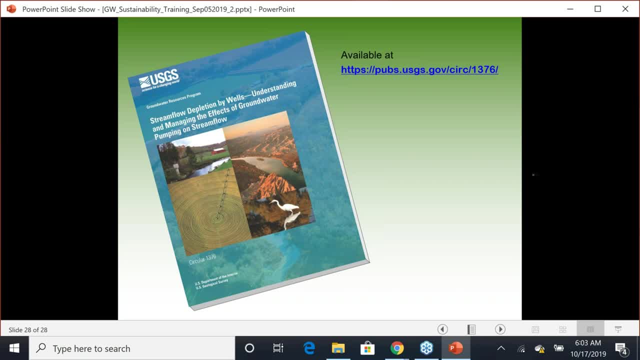 rescheduling this, this training, and for providing us with this insight on your experience and also the approach, which I find very interesting, coming from a sustainable development perspective, you know, and how do we merge the goals of water management with providing still the opportunity for human development, and how do we use a sustainability framework to make sure that we don't? 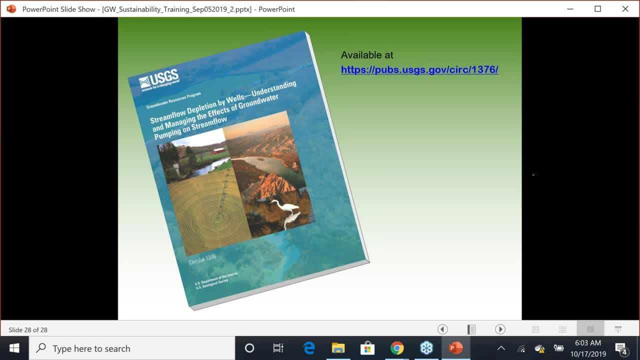 compromise sources that we have, not just in terms of pollution but in this case, into in the sense of extraction, and I think that for our research teams this is also very interesting, especially looking at your last light. and what is the role of scientists in making sure that we take up the sort of past research that has? 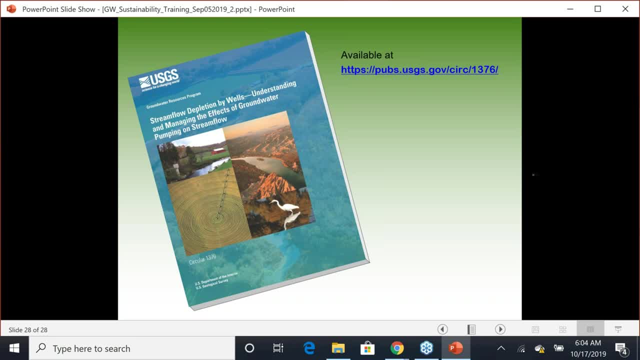 been done and past experience that has been done and make it ours and provide good insights in different other locations of the world and specifically for us in southern Africa. all of our projects are working in the Ramatua aquifer, which is between South Africa and Botswana. so yeah, I. 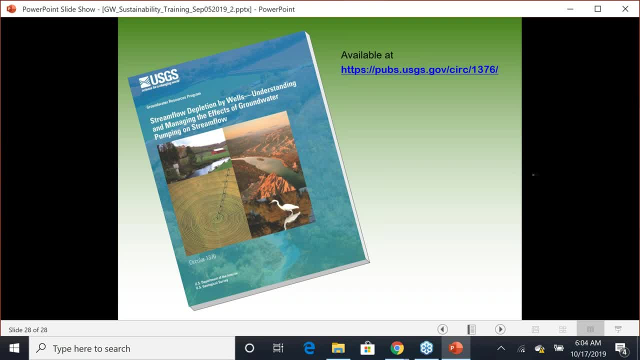 would like to thank you very much for this and I would like to open the floor to see if there's anybody who would like to make a comment on the presentation, provide insights from their own work or simply ask questions to Stan. Anybody brave, I heard a. 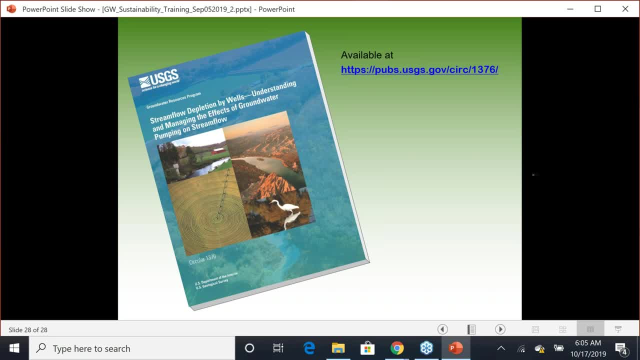 From Mark. he says he can't get his mic to work. Oh shame. Yeah, That's problematic. Yeah, because I can see that he's not muted, so he's definitely able to talk. Okay, Yeah, I went with the phone. 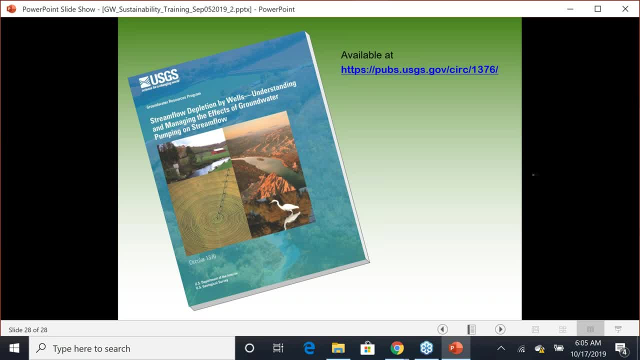 I just thought it would be more reliable. Thank you. I'm going to unmute Kevin Peterson, who's the research team leader for our project in the Ramatwa and the Shira River, so he can ask a question, as he's got to raise his hand. 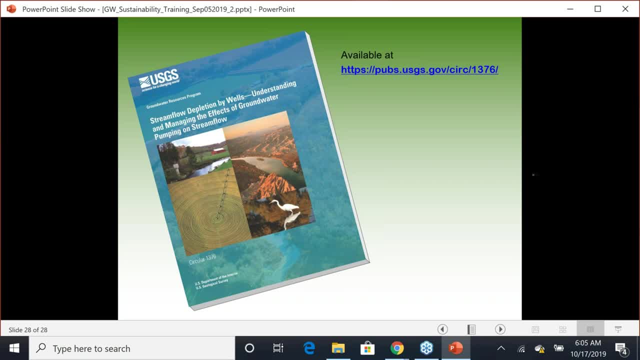 Thank you, Kevin. Can you hear me? Yes, I hear you, Okay, thank you. Thank you for the fascinating presentation, As sustainability is something that we struggle continually, you know, in terms of trying to understand. One of the biggest issues that we have is time and, for example, 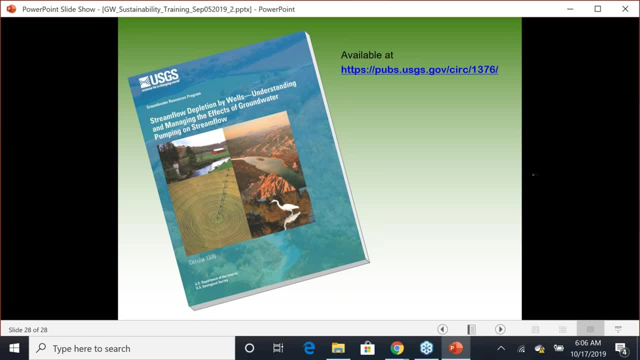 I'm now dealing, you know, around conflict between farmers, mines and municipalities in terms of exploiting, cost aquifers And, you know, as hydrogeologists we kind of defined or talk about 10,, 15,, 20 years' time. 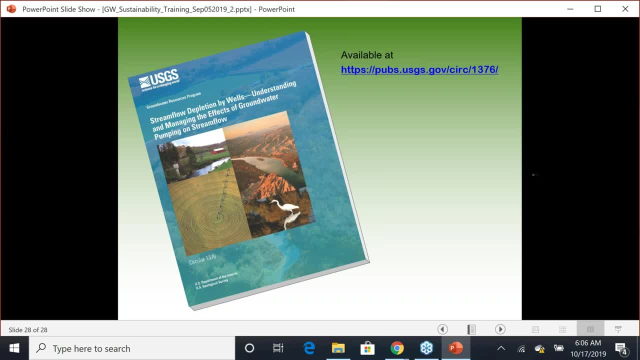 But no longer. So. I think that's a good question. Thank you. So normally in those type of conflict situations we don't have time to make the decisions that needs to be made, So the question goes around: you know, how do you get to a point of trying? 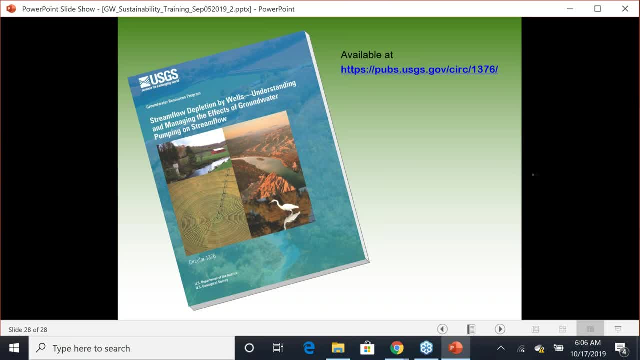 to define the acceptable tradeoffs between the various parties? and how do we deal with this whole time issue where we don't have the time to do the modeling studies, We don't have the time to do all the studies necessary to support our decision making? 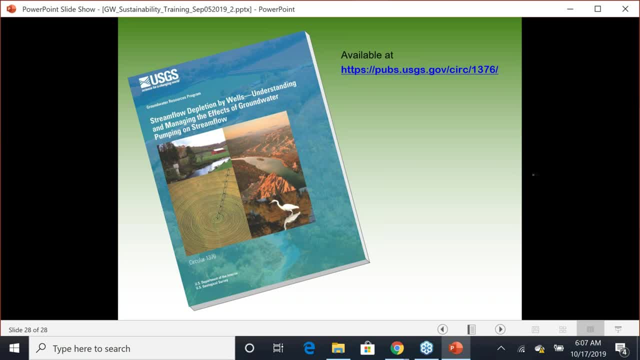 I'm just wondering: you know to what level- excuse me- you've had those kind of experiences where you're dealing with multiple stakeholders with expectations. Yeah, that's, I think, an issue that we all have. It's, as I understand it, you're saying you don't have the time to say. 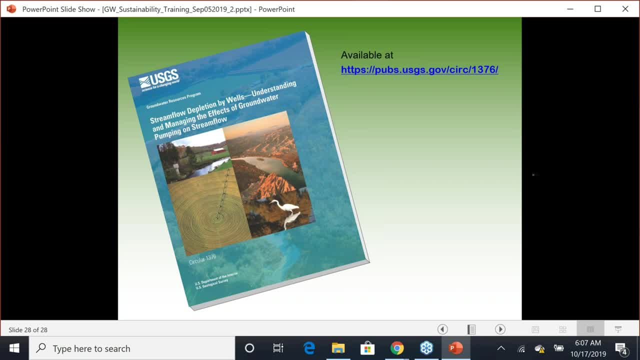 collect a long data series or to put together analytical tools. Is that right? Yes, that is correct, And what I'm trying to get to is: you know, how do you start defining what, what is acceptable tradeoffs between the various parties, and how do you move forward? 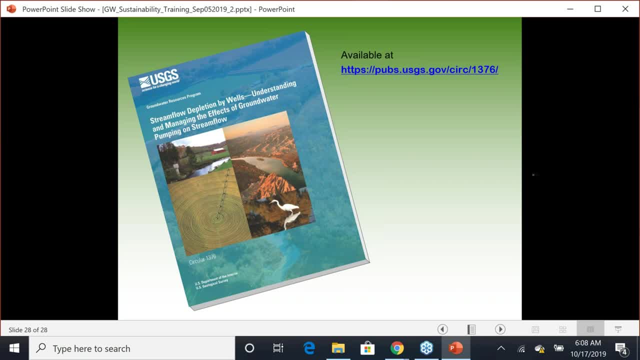 together in a partnership, as opposed to a conflict situation that normally results. Yeah, this is almost well here. some of those aspects would be at the state level. So groundwater management is done really at the state level and the USGS provides kind. 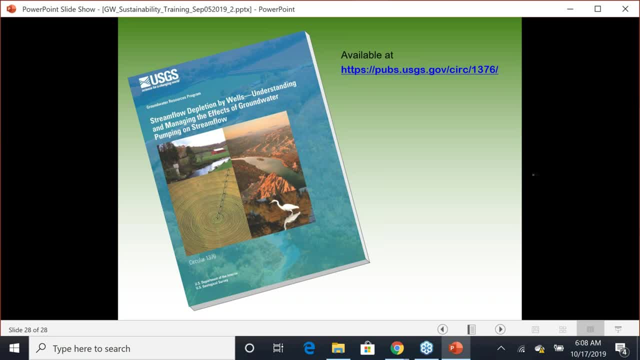 of some technical support, like databases, you know, and things like that, Yeah, Of, say, surface water flows and groundwater levels and things like that, or well databases, And then some states have their own databases. So here it's kind of a hodgepodge and some I think. so you might go to some areas of 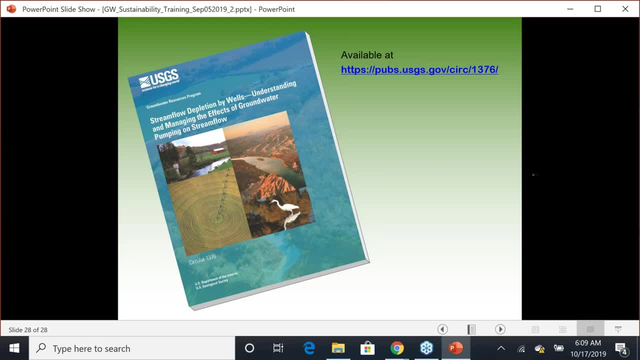 the US where, Yeah, you know that not much has been done because you know, like you say, it takes time and money. So I think you just have to start with whatever you can do. I'll admit that this kind of developing these databases and things like that, you know. 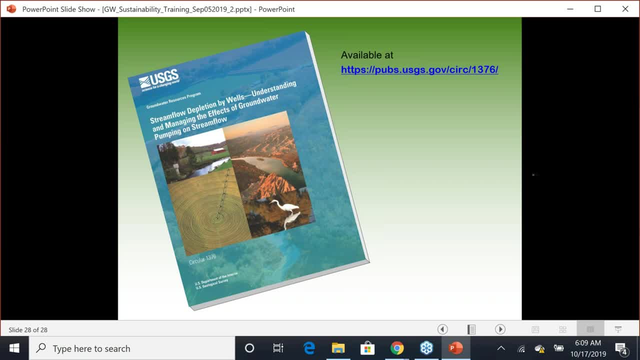 is. It's probably where you're at, It's not so much my expertise. It would be good if Mark could chime in, but I don't think he's able to. yet We have, Although I wonder. Sorry, Stan. 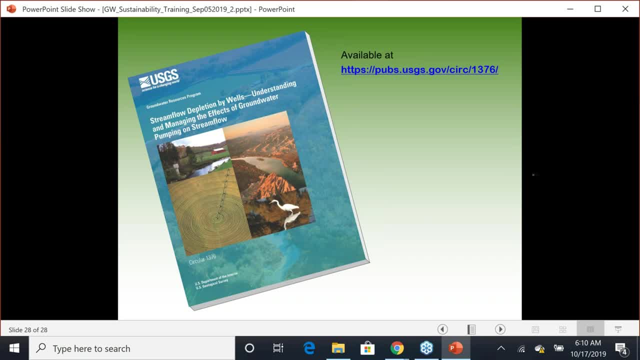 I wonder if he I'll, You have it, I'll. I'm trying to get Mark, So I am trying to see if he can chat, But in the meantime there is another question from Helen, who's a team leader for our Team. 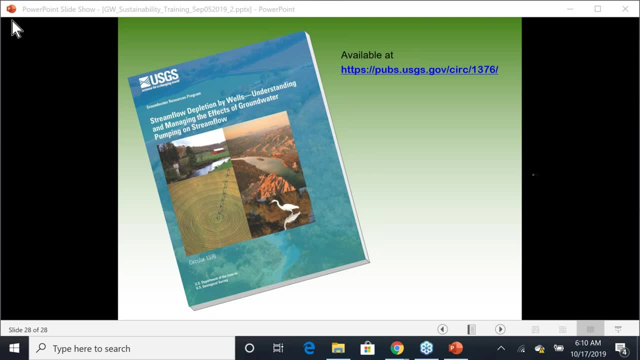 Four And she has a question that might be actually a follow-on to Kevin. so I'm going to unmute Helen, so she can ask the question to you directly, and then we can start a discussion on what happens when we have no data or very limited data. 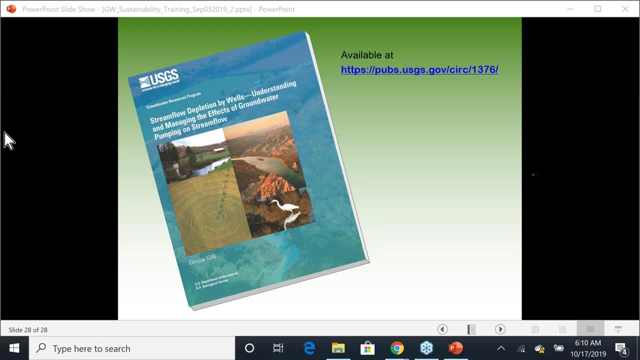 Oh, okay, So Mark is also here. So let me just unmute, Helen, and then I think we can have the conversation with Mark after she asks the question. Okay, Thank you, Helen. Hi, there, Can you hear me? Yes, 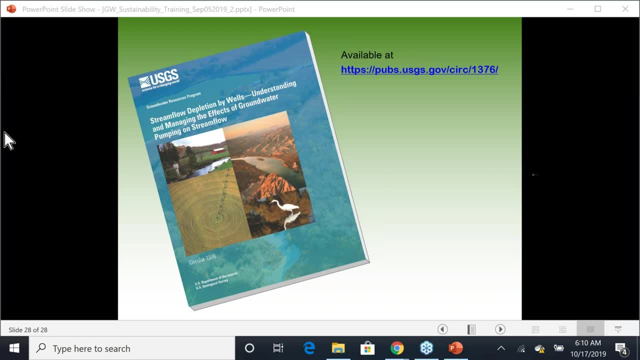 Yes, Thanks, Yeah, thanks. I really enjoyed the presentation and I very much enjoyed the Alley in Leak 2004 paper and referred to it many times, And we actually have referred to it in our current work on this project. We're specifically working on the Alley in Leak project. 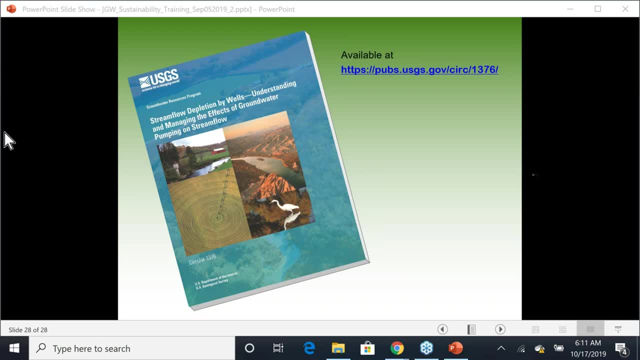 We're in the process of working on the Alley in Leak project. We're specifically looking at how we can kind of quantify those elements of capture and estimate the future dynamic equilibrium, possibly using big data analytics or different approaches rather than our kind of standard numerical groundwater modeling. 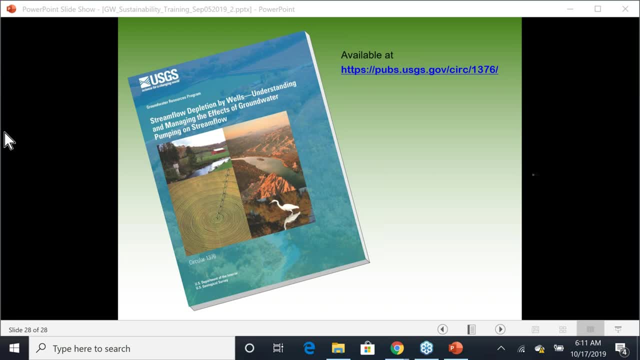 So we're looking at whether we can use artificial neural networks or machine learning models for estimating kind of those elements of capture And I wonder if you have any experience in that. And specifically our concern is that the artificial neural networks are not going to be particularly good at long term future predictions or predicting things that aren't seen in the training data set. 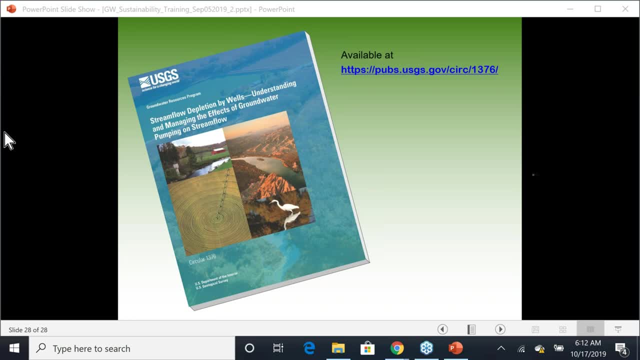 I wonder if you have any experience with that. I haven't done anything like artificial neural networks, but I am familiar with you, know analytical solutions for data, And I also try and steer people towards something called superposition or change model, So you can make like you may not have the time or the funds to make a calibrated numerical model. 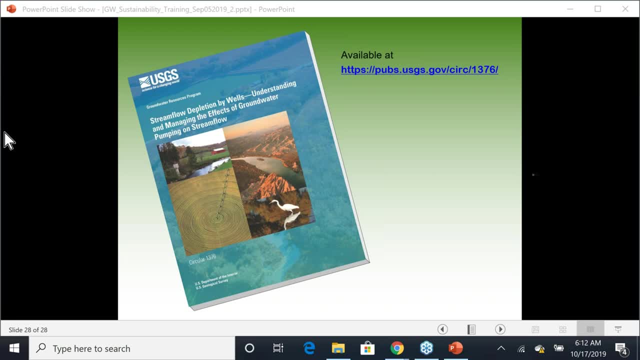 But you could do Something called a change model that incorporates the geometry of the system, for you know so there's a lot that we don't know about an aquifer, But the geometry, especially on the surface, is one thing we do know very well. 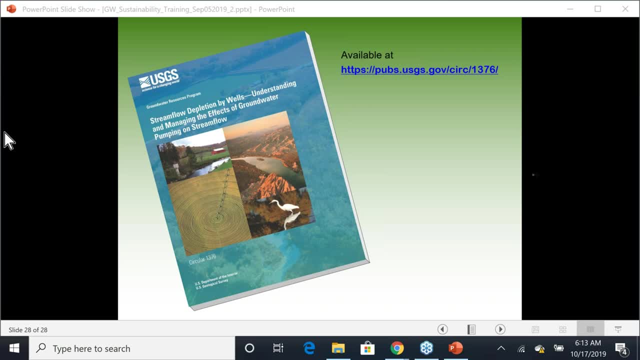 You know. we know where the rivers are, you know that are connected to groundwater, and we know where the wetlands are and things like that. So something that's very cheap and quick to do is a change model or a superposition model. 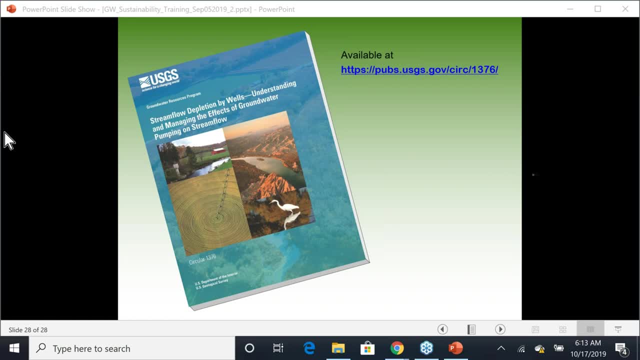 And they're usually not calibrated. They're kind of hard to calibrate, But the one good thing about this is that, of all those factors that I mentioned that affect the timing of capture, the single most important one is the distance from the well to the stream. 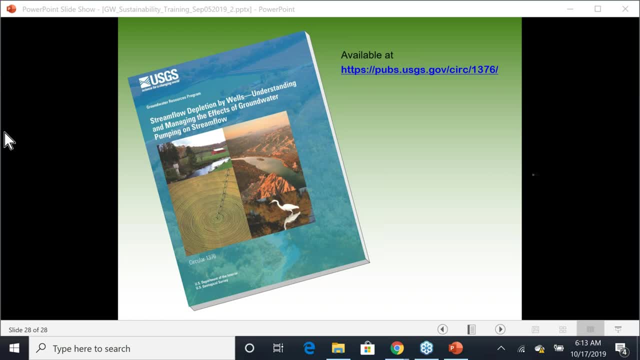 So in the analytical solution that distance term is squared, whereas, say, transmissivity and storage coefficient are just to the first power. So the thing that you know the best is happens to be the most important. And I've done, actually, quite a bit of superposition modeling along the Colorado River to look at which wells would be getting their water from the river that don't have a contract for water in the river. 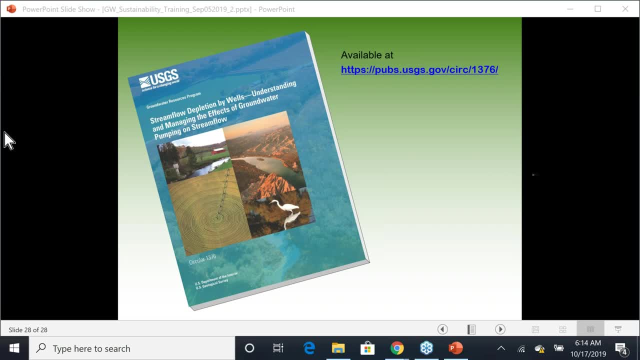 And I could provide References to USGS reports on that- and the analytical solutions themselves are can be handy, but you know they're restrictive, that you know the geometry of a straight river and aquifer boundaries have to be, you know, ideal for the analytical solutions to to really be correct, but they can still be useful. 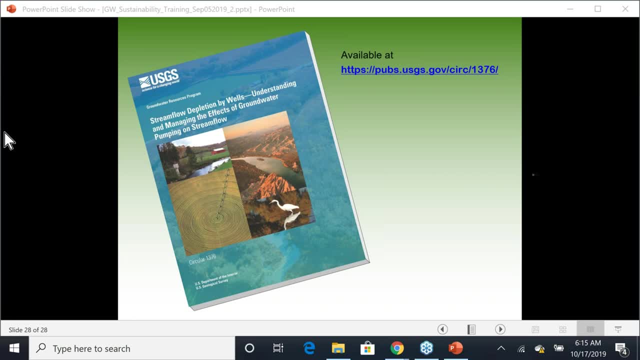 I don't want to discourage you from using them, but I've made capture maps using superposition models. I have some of those in report- USGS reports- If anyone's interested. Yeah, I mean, if you could share those with me on email, then I can put them up onto our Google LinkedIn and our Google Drive so that we can have them as reference for the project team. so that would be great. 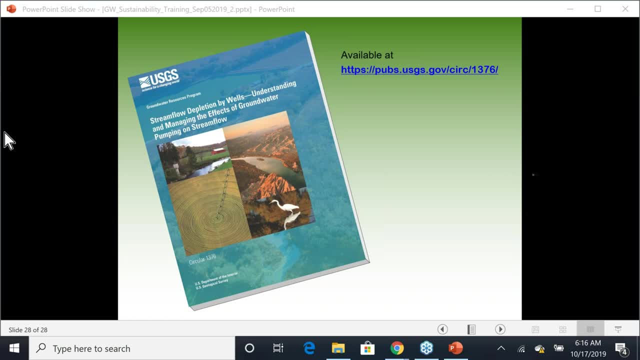 Thank you, Sorry. the geometry model we're referring to. is that related to the evapotranspiration modeling that Gabriels and I talked to us about last week, Yeah, or is there something else? I'm just trying to understand. It's for my own curiosity. 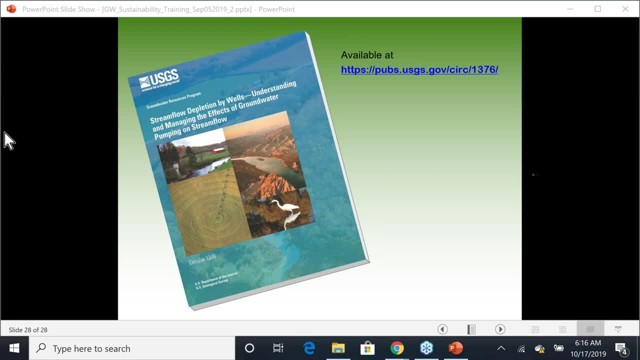 Hello, Was that for me? Yeah, Oh, okay, I didn't see Gabel's talk, So So he's using satellite imagery and whatnot to estimate evapotranspiration rates. Is that correct? Yes, it is, It is. 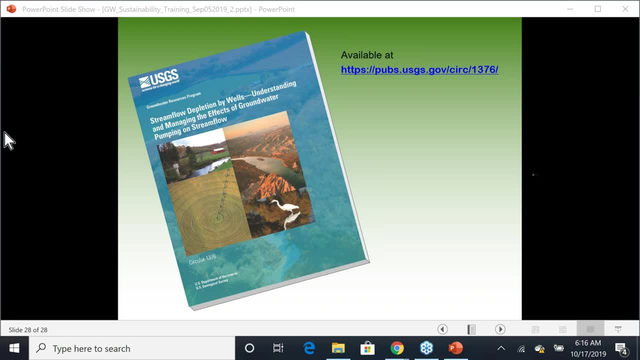 But he also mentioned something around like- again, please bear with me, I'm not an engineer, nor am I a geologist, so I'm just trying to make sense of things in my head. But he also mentioned a question of geometry. 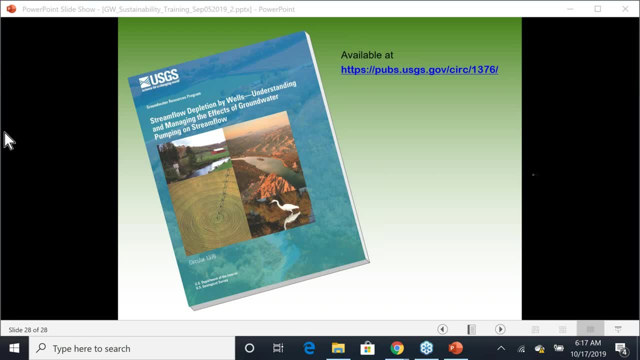 and using geometry to sort of triangulate and verify the information that one gets from evapotranspiration. So I was just curious what you were talking about with one of those elements of triangulation of information. Okay, Okay, So he's using the geometry of the ET areas. 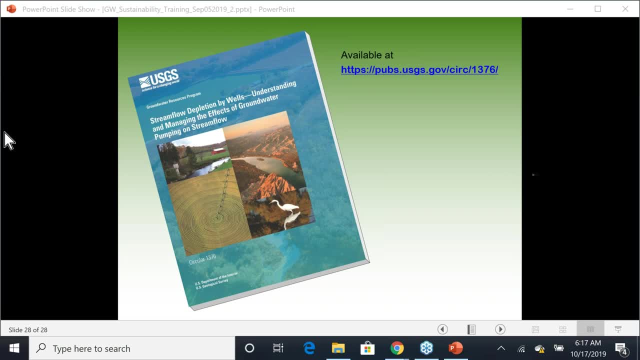 If I understood, Yeah, yeah, If I understood, Just bear with me. Yeah, So with regard to you know what I'm talking about: capture. So we're talking about a change. So he might estimate the overall rate of ET for a particular area. 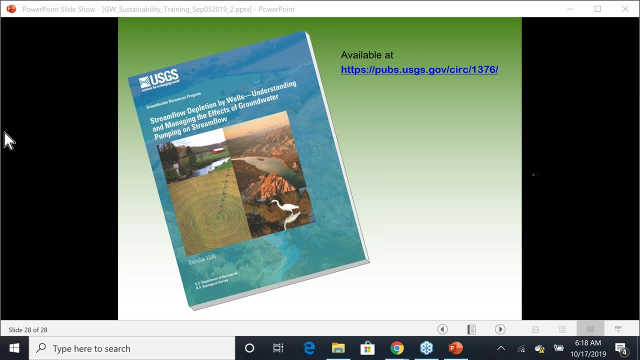 And then what I would be concerned with is: how does a well pumping affect that rate? Because we know that the deeper the water table goes, then the less will be transpired. So you know, we would use the rates that he would estimate. 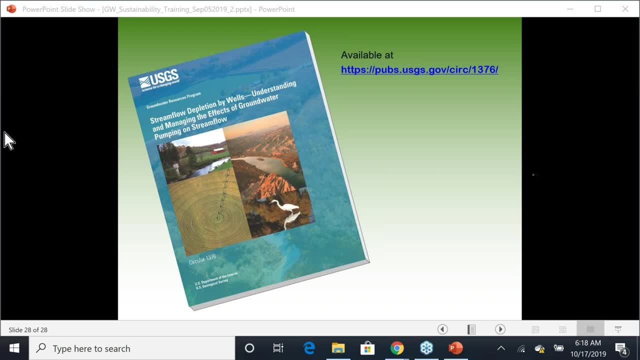 and the areas that he would estimate. importantly say, in a model to calibrate, We would try and simulate the right amount of water, leaving the system at those locations, locations, and then our models would try and predict how that would be reduced. let's see. 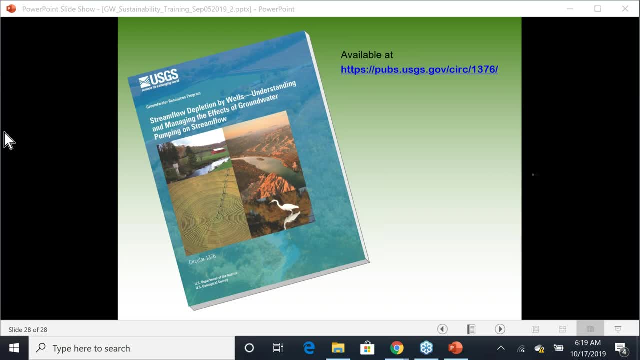 I'm not sure what more I could say about that. oh, I just want to say that we have this very simple function that we're using most groundwater models where there's a linear relationship between depth of water and ET. so we say that when the water goes to a certain level, ET ceases and then 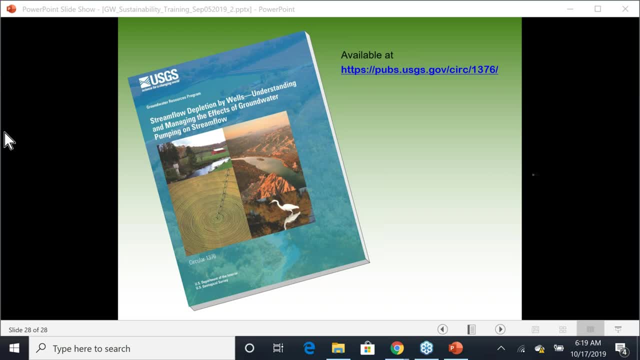 on the other end, ET is at its maximum when water levels at a certain point. so we have this kind of piecewise linear function. so it's a very simple approach in our groundwater models. that may not be strictly realistic, that may not be really linear, but we treat it as such, especially in our, you know, basin scale or more regional. 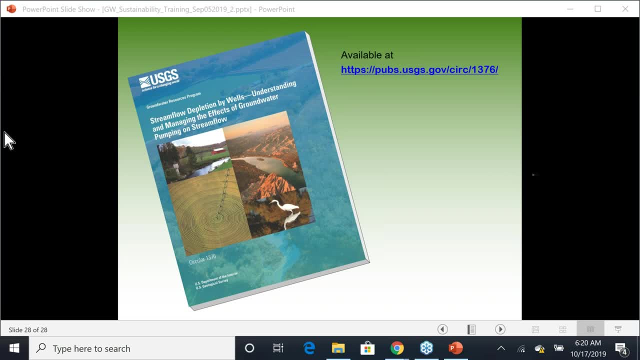 groundwater models, it's probably good enough. so our approach is, I'd say, somewhat crude. and there are a little more sophisticated ET packages for the models, that there's one called riparian ET that you could have, for instance, simulate anoxic conditions when the water level gets up into the root zone. then you start to kill off the plants. 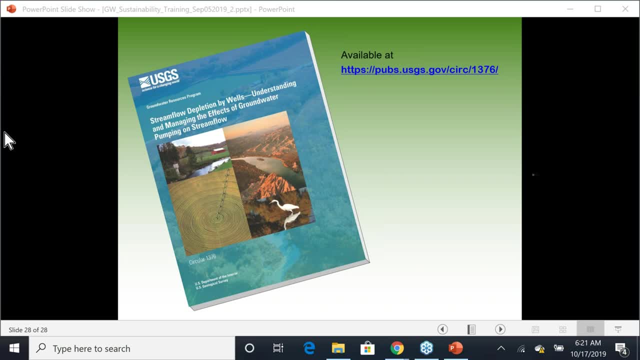 real detailed studies of riparian areas. but, um, anyway, thank you so much. yeah, this this is Mark. is there any chance you can hear me now? yes, we can. yeah, I'm using my phone now. sorry about that. yeah, so, Clara, do you want me to make a couple of comments? finally, 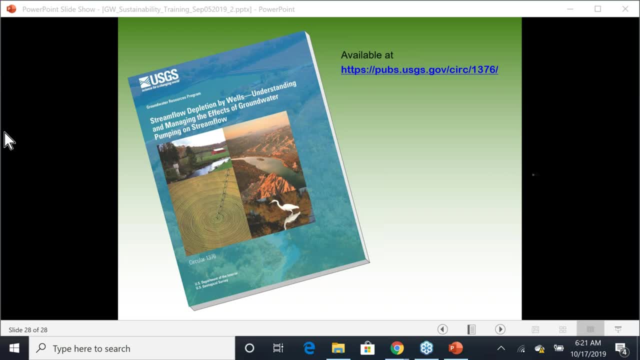 close, otherwise we running out on our webinar time. oh, that's right. yeah, you're gonna potentially run out of power too. huh well, anyway, I just wanted to uh relate. first of all, I apologize for uh not being on the beginning of the call. I joined about 10 minutes later. first of all, I want to thank Stan. uh, kind of give a re-entertainment. 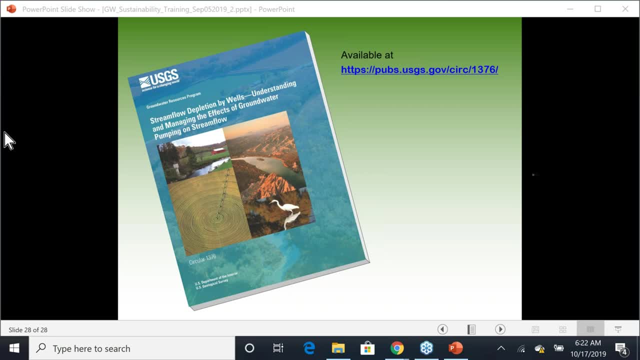 Stan is one of the intellectual powerhouses in groundwater in the USGS and I'm so pleased that he was able to join us and give some of share some of his wisdom. I've taken a lot of classes in groundwater over the course of my life, but I learned more from working together with Stan. 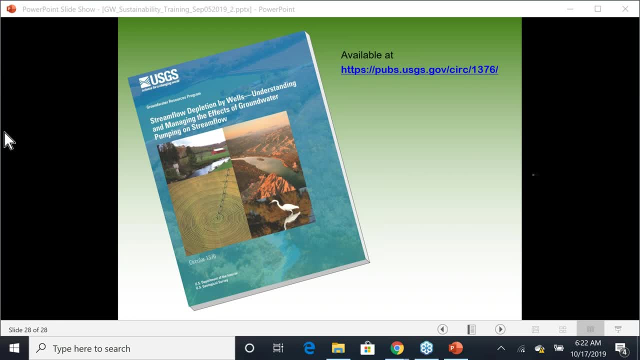 over the course of 15 years and I guess even longer than that- about how groundwater really works, and so I'm glad he was able to share some of his knowledge with with the team. I think a lot of these principles are really foundational in the sense that when we start thinking about how 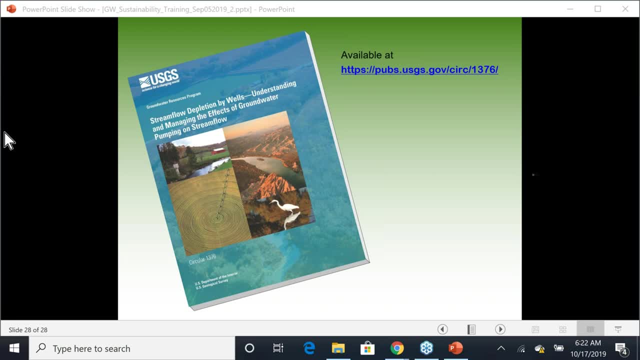 do you make use of a an act for whether it's a trans boundary act, for any other act? for you know, some of these principles need to be really considered as, as you begin to plan, yes, there's always a lack of data. seems like going back to Pearson's question. 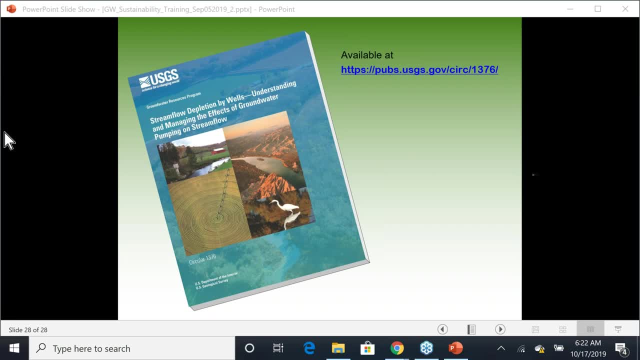 but understanding these principles can also help you understand. you know, maybe you don't have the precise numerical answer, but at least you understand that you know. for example, pumping even from a well that's a distance away from a stream can eventually in time affect the stream flow, so on. sometimes a very valued stream like the San Pedro, or certainly every place, has ecosystems. 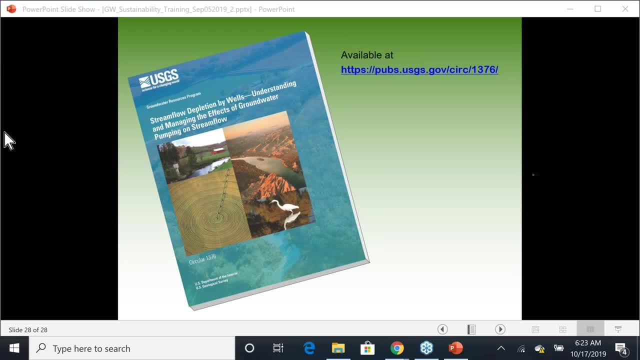 that are highly valued. so, again, this will end up concluding our regularly scheduled series of the seminars, and there may be more in the future if specifically requested, but right now this is the last one we have scheduled and anyways, ironic that I would have so much trouble on the last one, but anyway, anyway, thanks. 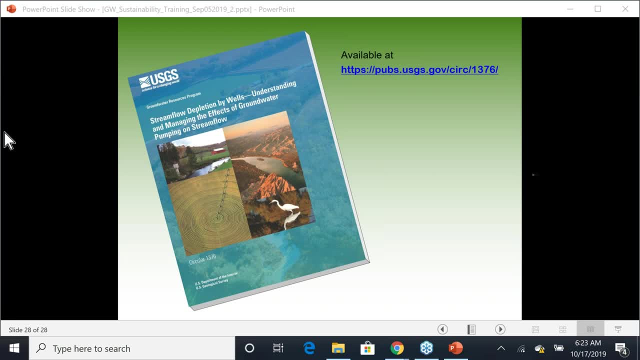 to to Stan. thanks, Clara, for making the organization happen. I'm not sure what else to say at this point, with only a couple of minutes left, about complex principles of groundwater, but I think these are very foundational and I'm glad we were able to cover them. Stan and thanks. 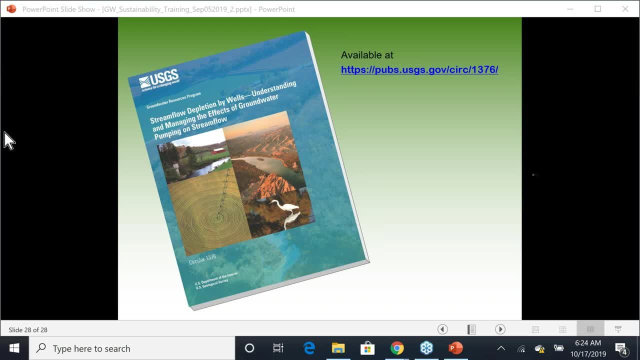 for getting up so darn early down there in Arizona. I'm glad to do it, thank you. thank you, Stan and Mark. I think what we can also say is that you, we're going to organize another USGS travel to southern Africa, where there will be a face-to-face seminar with you, mark. so hopefully. 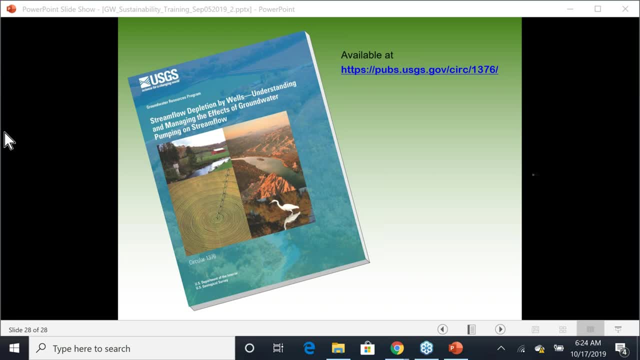 next year. that will happen and I'll see you next time. Thank you so much for joining us today and we hope that this will happen and we'll work towards making that happen. in the meantime, we're going to share with all the people who participated in this seminar form to ask us for opinions and suggestions to improve our series of webinars as we prepare for the IBM Research Africa crash course on big data analytics and then possibly another course on transboundary water governance next year. so thank you everybody, thank you to USGS for this first webinar and I hope to see you next time. 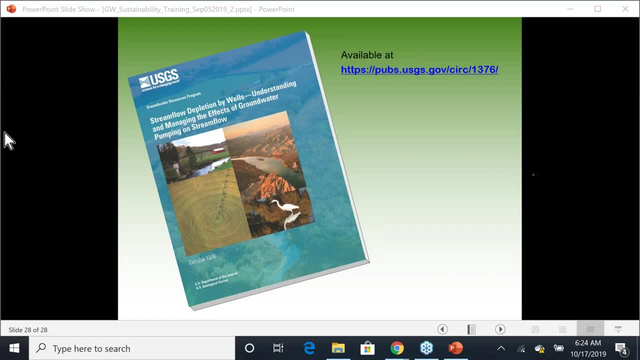 trial of webinars that we've had and seminars, and thank you to everybody who attended over the course of the past three months. I wish you all a good afternoon and, for those of you in South Africa, watch out for the load shedding. Bye, bye.